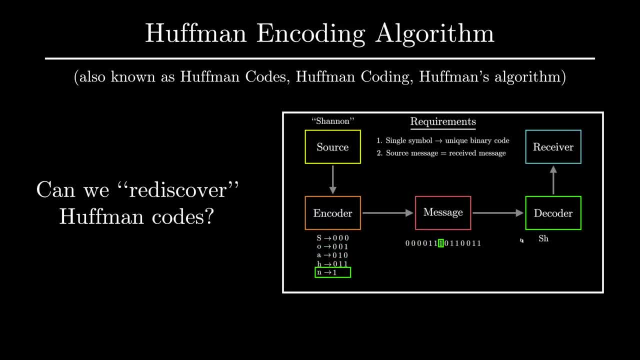 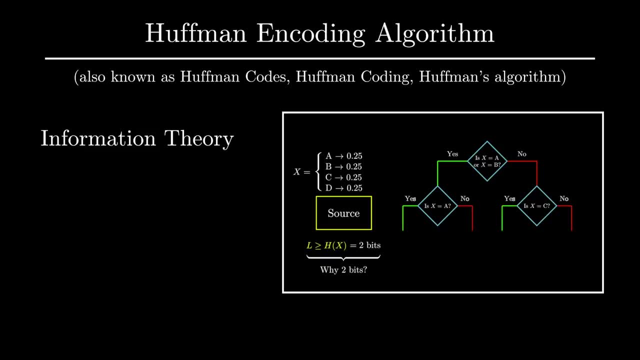 a journey into the process of how we might rediscover this algorithm On the way. this gives me a good excuse to dive into the fundamentals of information theory and some of the key ideas that led to modern techniques in data compression. I think by the end of the video, no matter what. 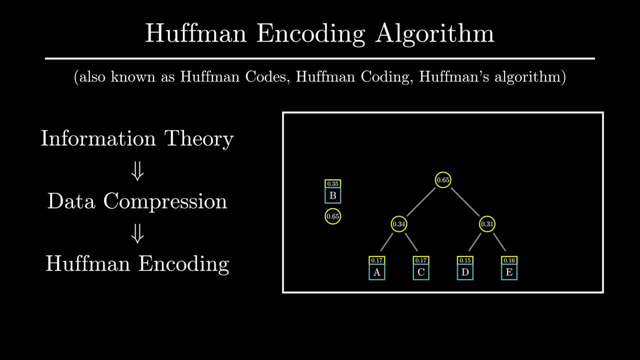 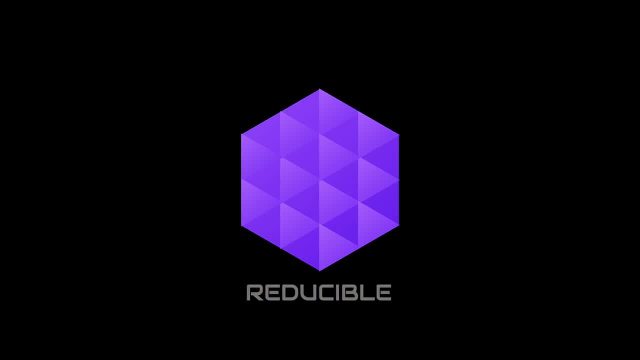 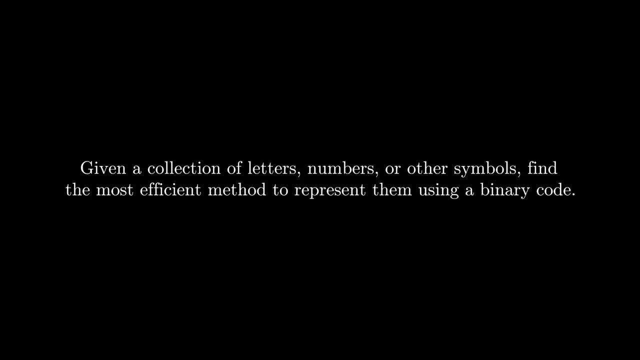 your familiarity is with Huffman encoding. you'll get something meaningful out of this journey. So let's get started. When we are faced with an open-ended problem, it helps to have some tools in our arsenal. to break down the core problem. To formalize the problem, let's introduce a common setup. 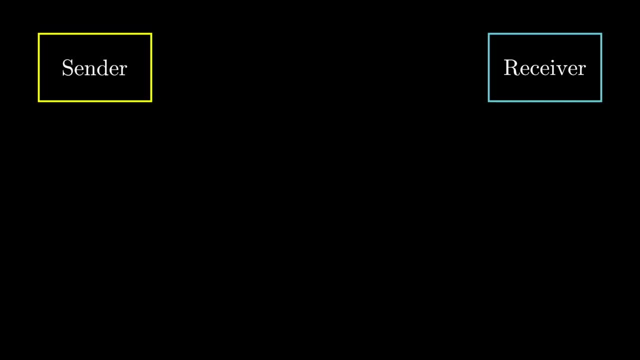 We're going to define a communication network where we have a sender of information and a receiver of information. We often refer to the sender as the source In our network. the source wants to transmit the information to the sender and the sender wants to transmit the. 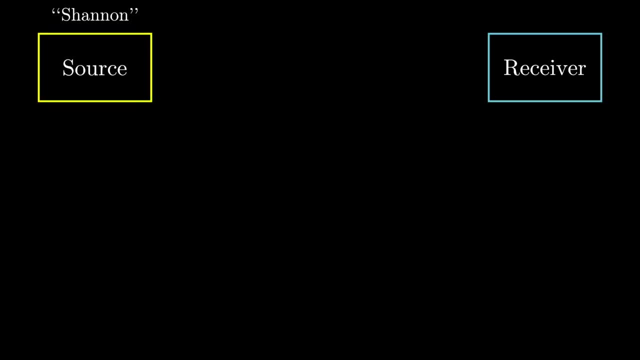 original message. The only means of communication in the network is through bits, so the source has to find some way to encode the message according to some mapping between symbols and binary codes. Before the message gets to the receiver, the encoded message must be decoded. 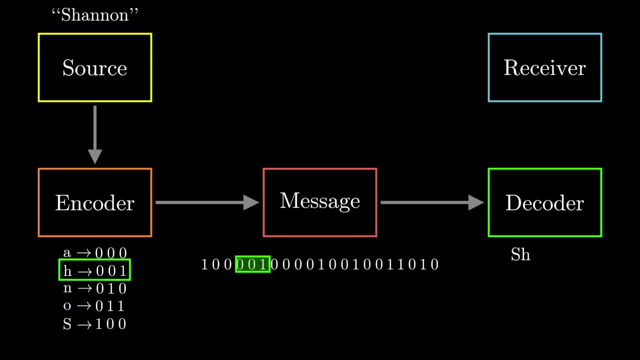 so that the receiver can get back the original message. There are a lot of moving parts in this setup that I want to make sure we don't take lightly. We need to be able to get the original message to the sender so that the receiver can get back the original message. 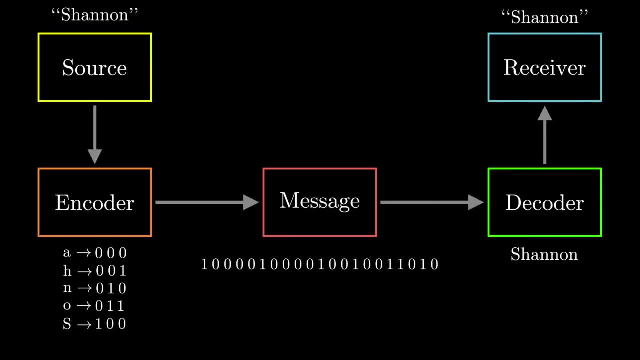 be aware of all parts of the setup, but compression specifically focuses on the encoding step. There are tons of ways we can encode a message- some ridiculous and some super clever- But the fundamental goal of an optimal compression algorithm is to find an encoding that uses. 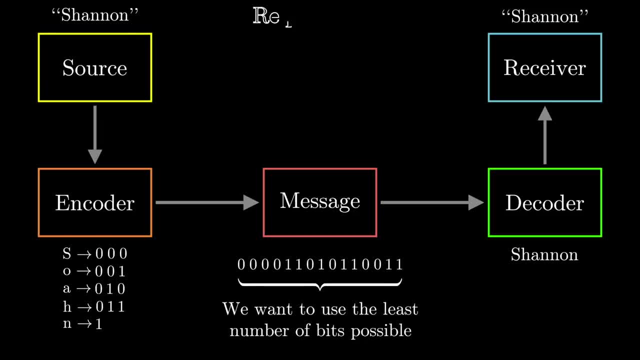 the least number of bits possible. There's some inherent requirements here. The first is that each symbol must be mapped to a unique binary code. This is a constraint of the problem Huffman was trying to solve, meaning that an encoding scheme that maps a combination. 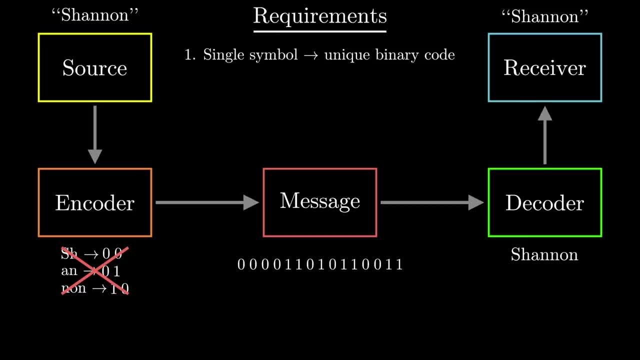 of symbols to the same binary code is not valid in this context. The next constraint is that the receiver must be able to decode the exact original message. We can't lose any information in this process. Notice that in this particular encoding, if we try to reduce the number of bits, 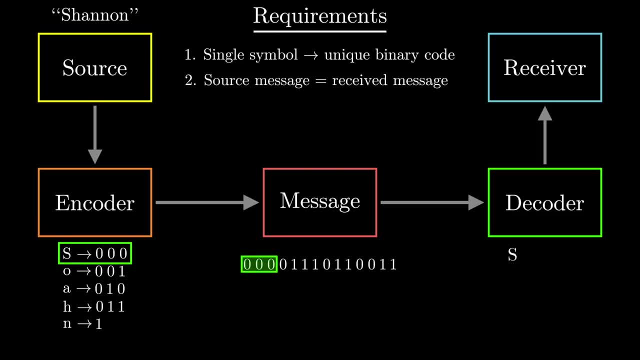 by randomly removing a bit from the message, we end up losing the original message. This constraint is often referred to as lossless data compression. The third major constraint is that, given an encoding scheme, the decoder must be able to unambiguously decode the original message. This constraint is often referred to as 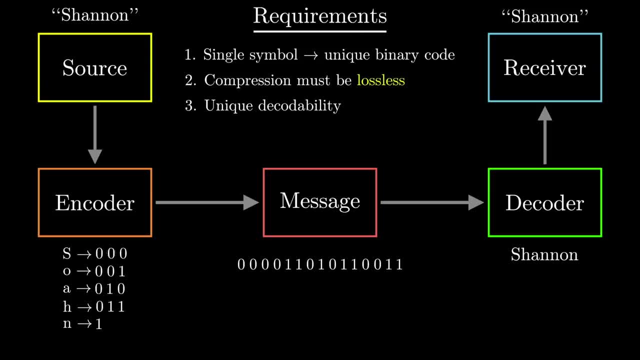 unique decodability. Take this slight modification to the current encoding scheme where we try to reduce the length of our message by one bit. The problem here is it's impossible for the decoder to figure out which message is sent. This is an example of an encoding that is: 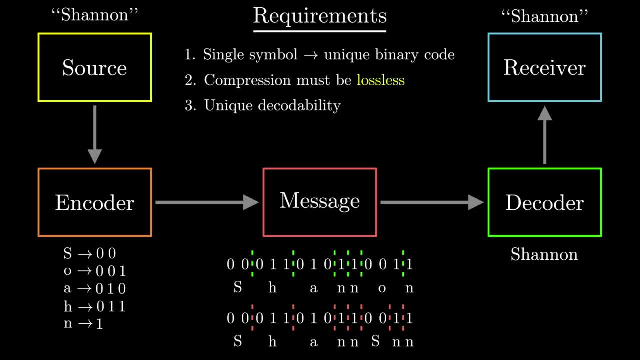 not uniquely decodable. The solution that Huffman created satisfies all these requirements, and he also proved that there's no better encoding scheme given these constraints. By the end of this video, we'll see why this is true, but to get there we're going to need some. 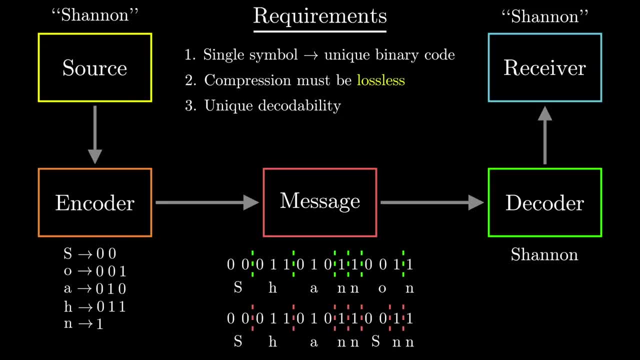 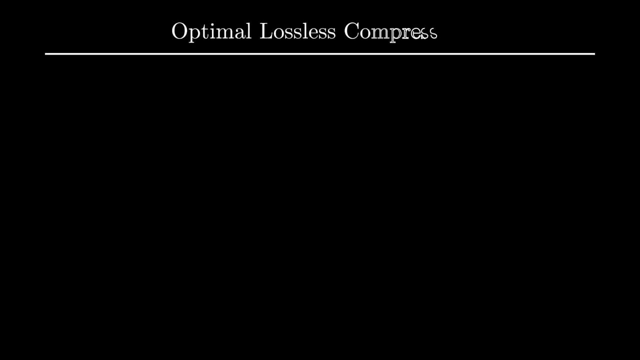 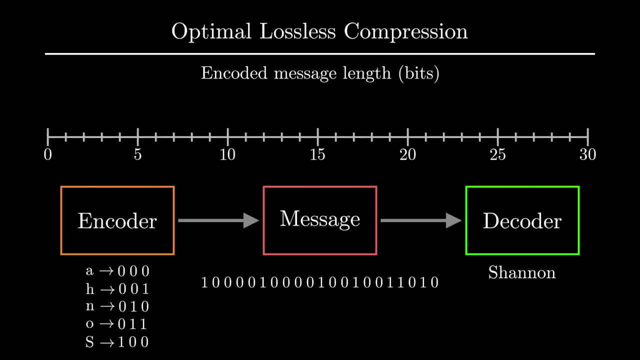 information theory To introduce that. let's focus a little bit on the lossless compression constraint and its deeper implications. If we think about what we need in an optimal lossless compression algorithm, it ends up being fundamentally a balancing act On one side. we have to be careful. 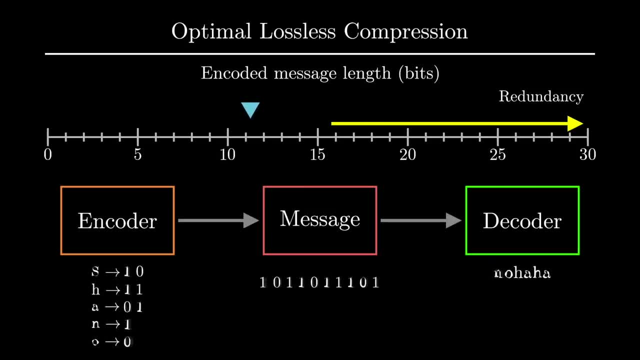 about not using too many unnecessary bits, but if we use too few bits, we end up losing information from the original message. This brings up an interesting question. It seems like there must be a limit on the amount of compression possible that still retains the original message. 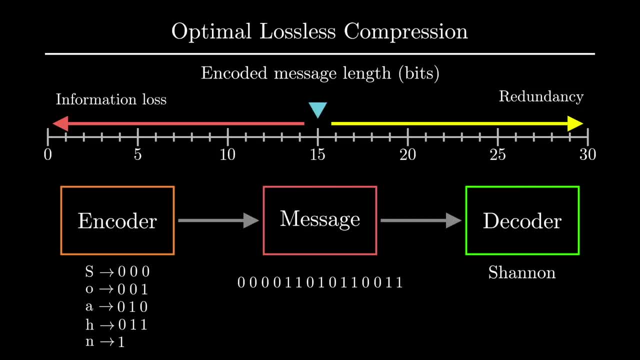 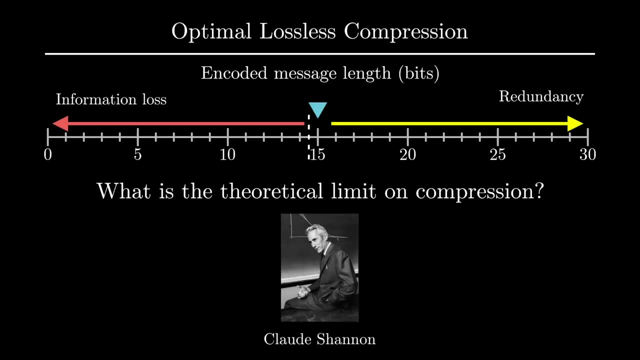 In this situation. it turns out that if we try to compress our encoded message to less than 15 bits, we are guaranteed to lose some information. But what is that limit in the general case? That, my friends, is the exact same question Claude Shannon asked in this exact context. 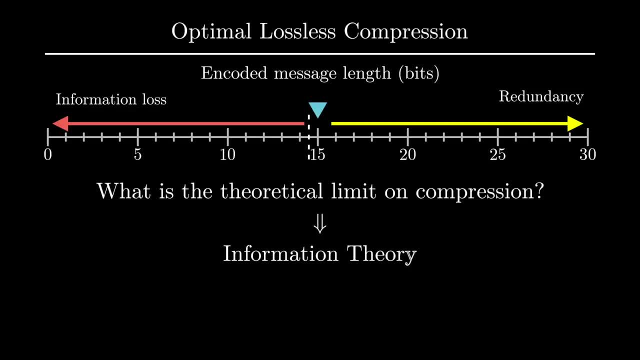 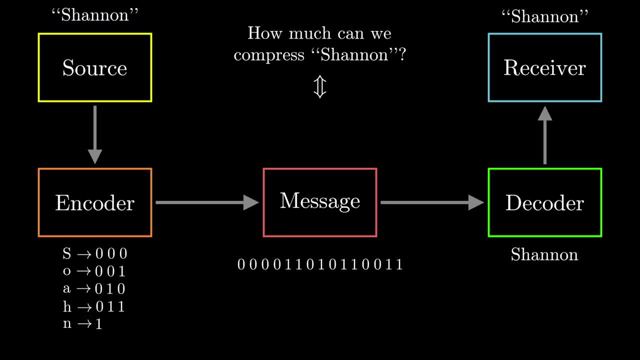 and the answer is the foundation of information theory. In a sense, asking about the limit of how much we can compress a message fundamentally is also asking about how much information is contained in that message. The question now is: how do we objectively measure information? 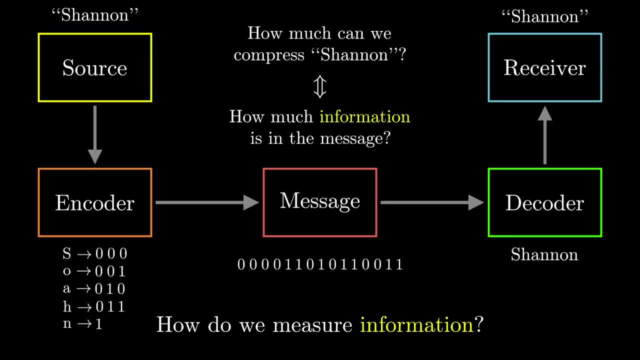 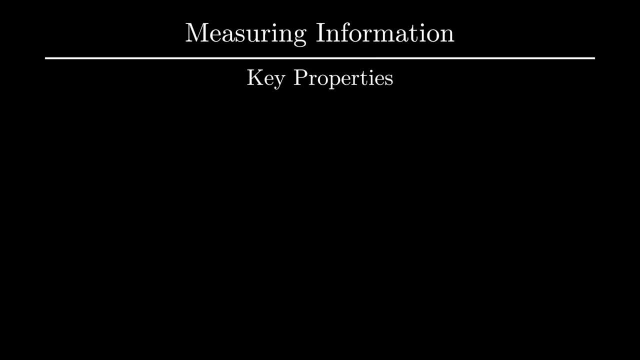 This is pretty vague, but let's play around with some ideas. Suppose we wanted to create some metric for measuring information. What properties would we want? One thing Shannon realized while thinking about this problem is that information is somehow related to uncertainty. For example, suppose I gave you the following 2 statements: 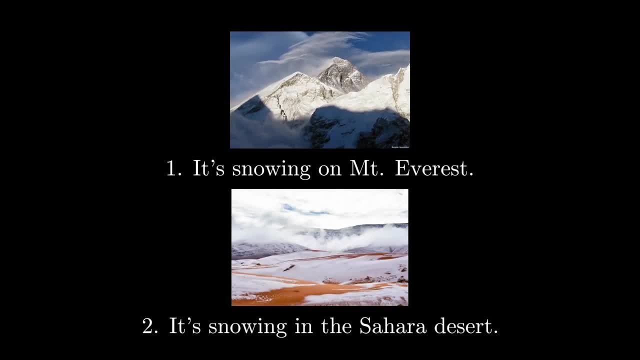 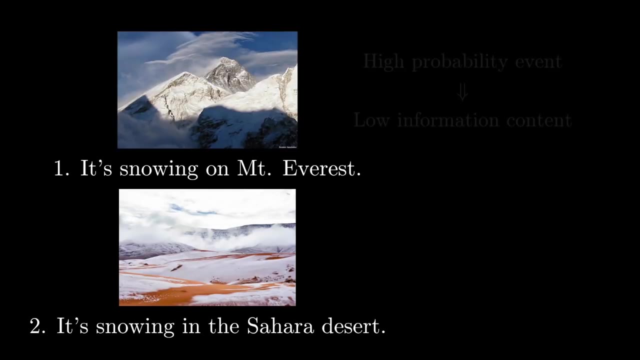 It's snowing on Mt Everest and it's snowing in the Sahara Desert. Which one provides more information? I think we can agree that number two is the expected answer here. Finding out it's snowing in the Sahara Desert is way more surprising than finding out it's. 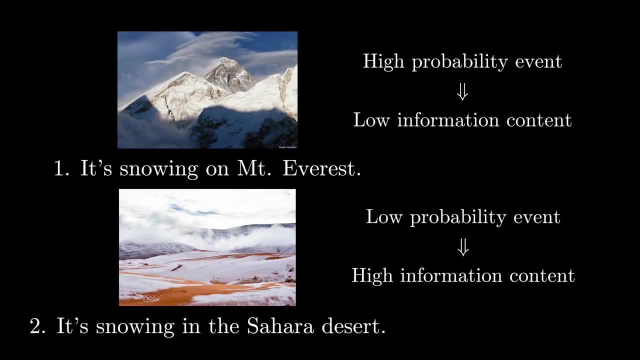 snowing on Mt Everest and that, in a sense, should give us more information. Thought experiments such as this one was a good indicator that the probability of an event occurring is related to the amount of information tied to an event, Specifically, a key property Shannon realized was essential to appropriately defining a measure of 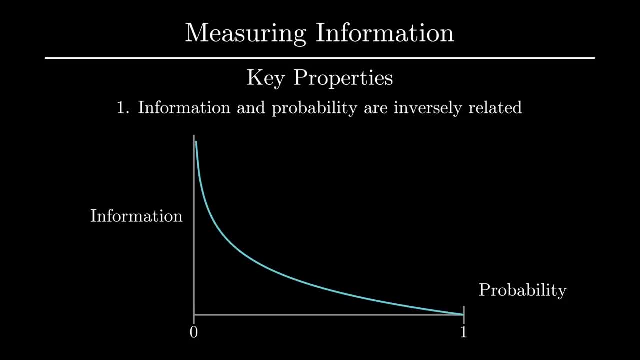 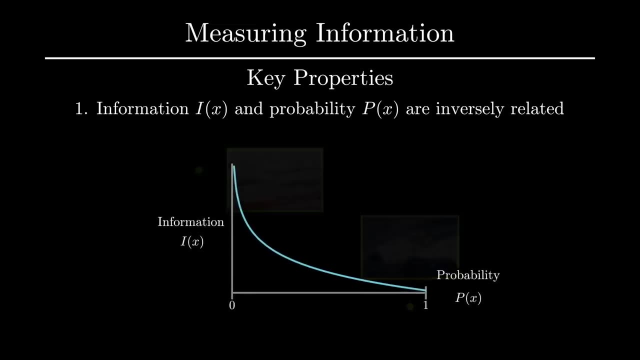 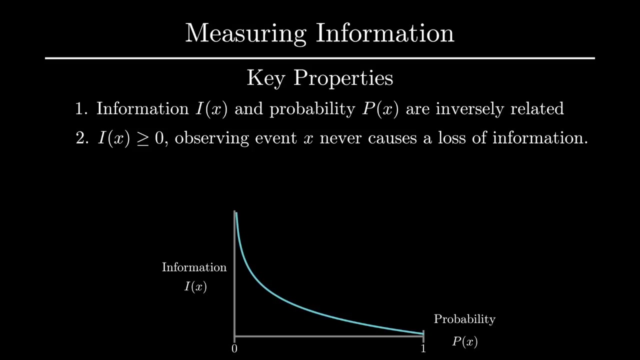 information is that information is inversely related to probability. This was one of four key axioms for Shannon's definition of information. Let's denote this information metric as i, where x is some event that occurs, with probability p. Any metric for information should be non-negative. Observing an event should never cause you to lose. 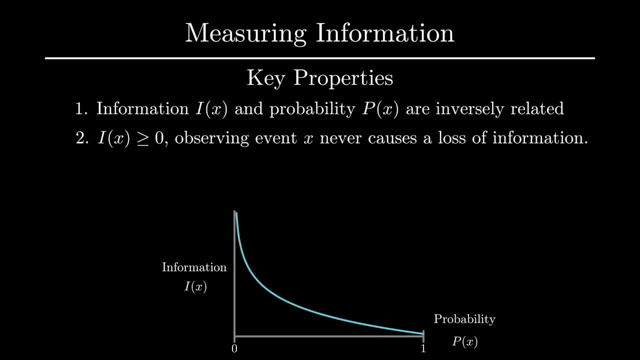 information or increase uncertainty. The third key property is that an event that occurs with 100% certainty yields no information. And, lastly, if two independent events are observed separately, the total information from these observations should equal the sums of the information of each of the events individually. 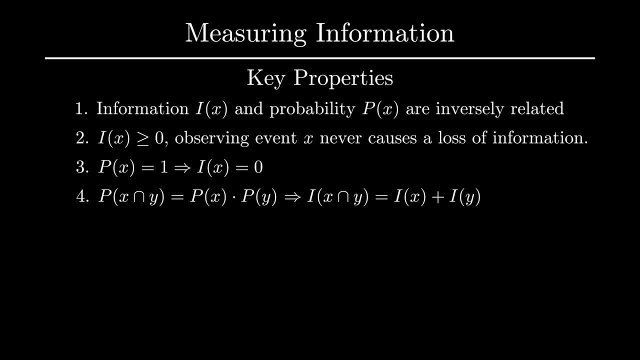 Any metric for information should be non-negative. Observing an event should never cause you to lose information or increase uncertainty. So the question now is significantly more precise: Is there a set of functions that satisfy these particular properties And in fact it can be proven that the only set of functions that satisfy these four properties? 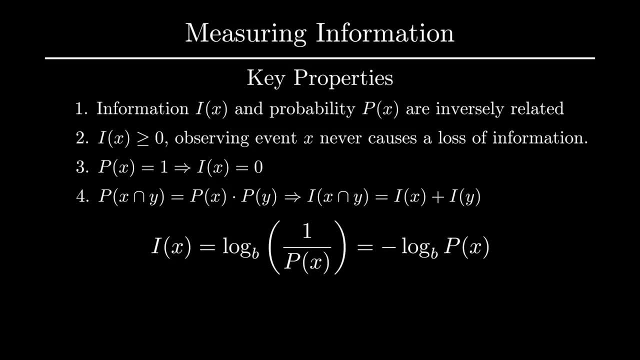 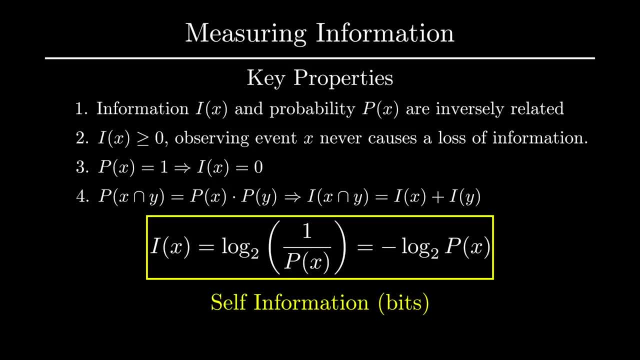 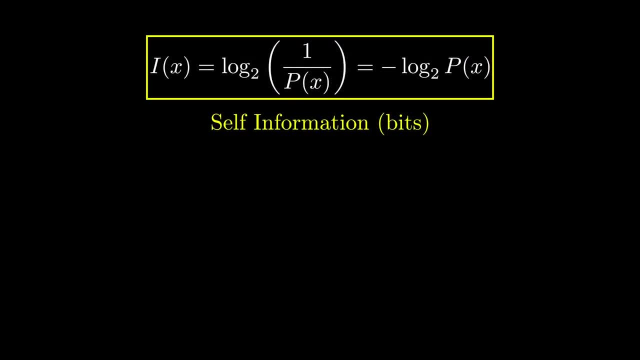 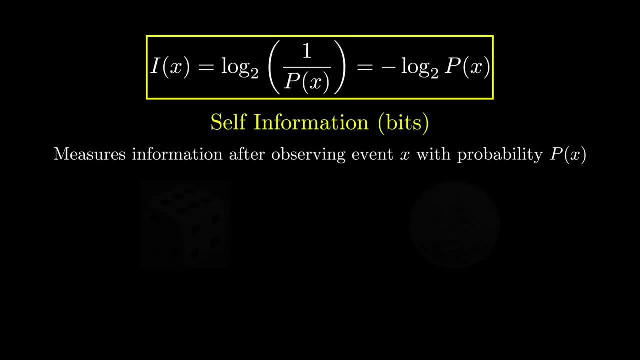 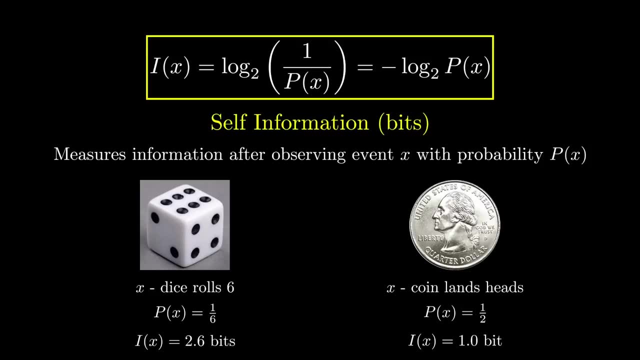 x that has a defined probability associated with it. For example, if you observed a balanced dice roll was 6, we could say the observation yielded 2.6 bits of information. A coin tossed landing on heads gives one bit of information, But self-information is only the start of. 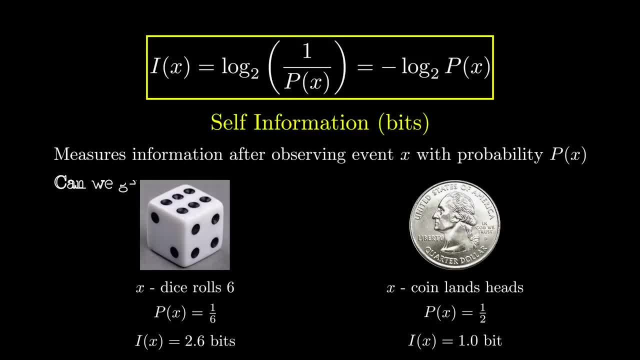 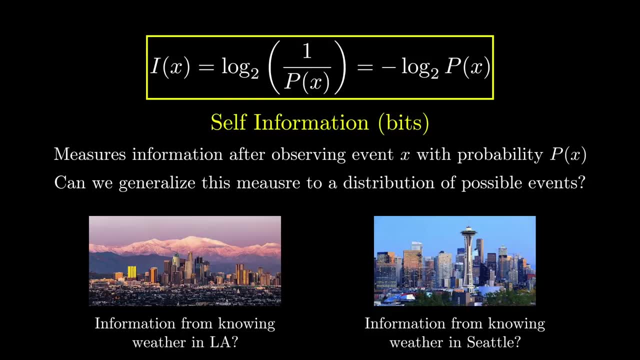 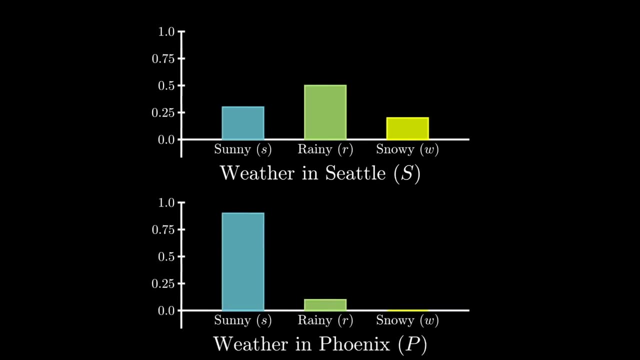 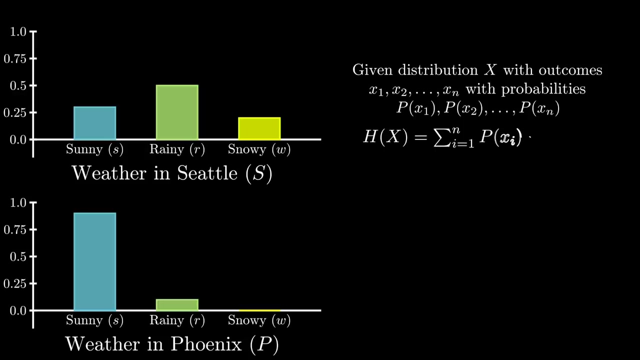 understanding how to measure information. One of Shannon's biggest contributions was extending this notion of self-information to general probability distributions. Suppose I gave you the following distributions for weather in Seattle versus weather in Phoenix. A natural extension for self-information for a general probability distribution is to just take 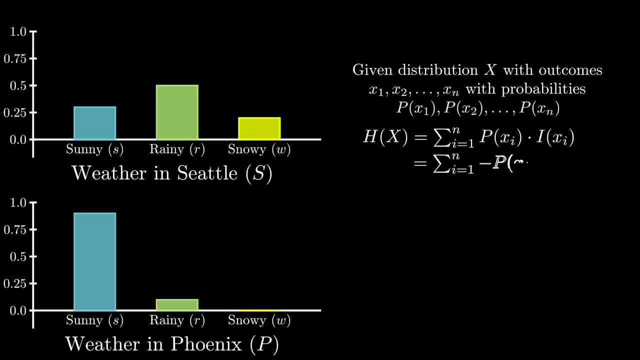 the weighted average of the self-information of each event. Shannon called this quantity the information entropy of a distribution. Here are entropies for our weather distributions. A nice intuition on entropy is that the more unpredictable a distribution is, the higher the information entropy is for the distribution. 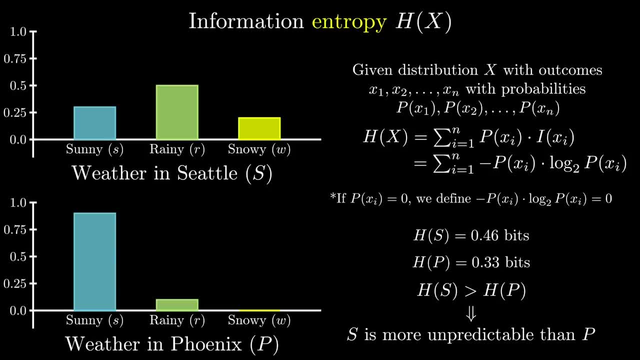 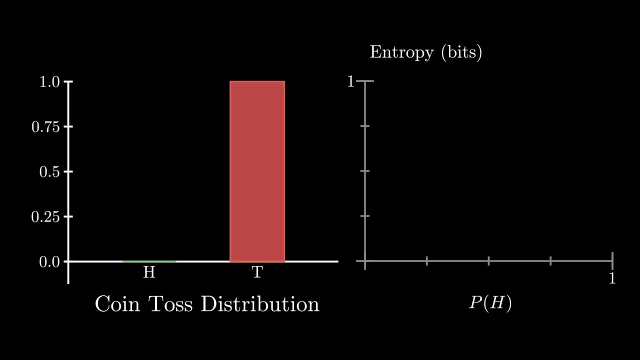 You would expect the average person in Seattle to check the weather more often, since it's harder to predict than the weather in Phoenix. so this matches the intuition. The best way to see this in action is by looking at the entropy of a distribution describing a biased coin, Among all possible probabilities of getting heads on a biased coin flip. 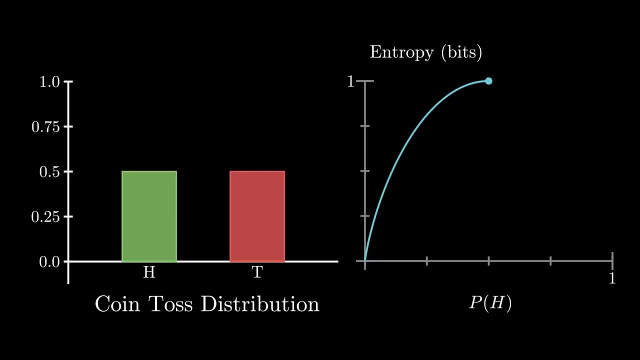 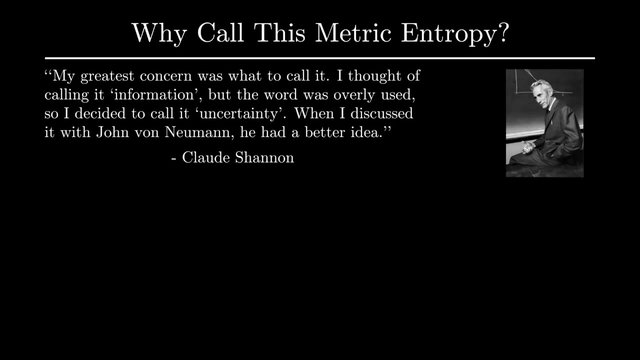 the entropy is maximized when each outcome is equally likely, which is when it's hardest to predict what the outcome of the distribution is. Some of you may be wondering at this point why Shannon called this measure entropy. It seems a little random. Turns out that Shannon actually had some trouble naming it. 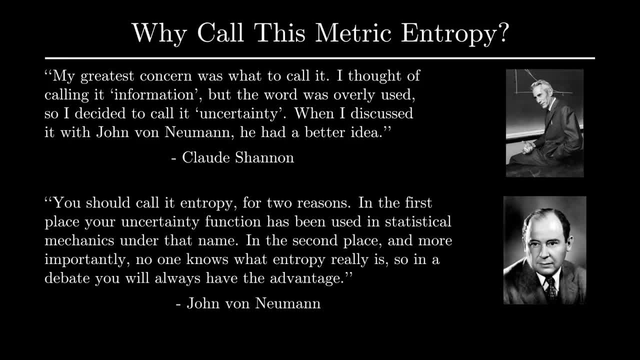 The origin of the name comes, with some help, from John von Neumann, another huge figure in computing. When Shannon asked him about what he should name this quantity, von Neumann mentioned that the word entropy has been used in a similar context in statistical mechanics. The answer is the same, but it's not the same thing as the word entropy. But the more 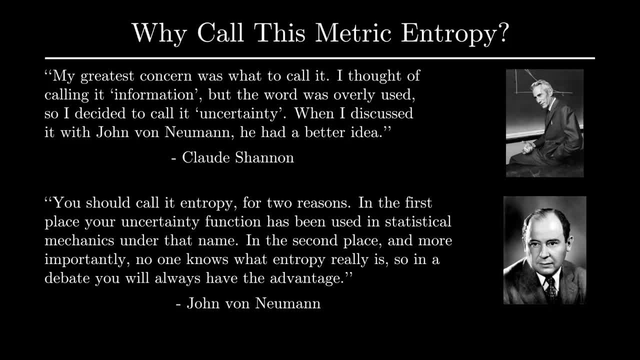 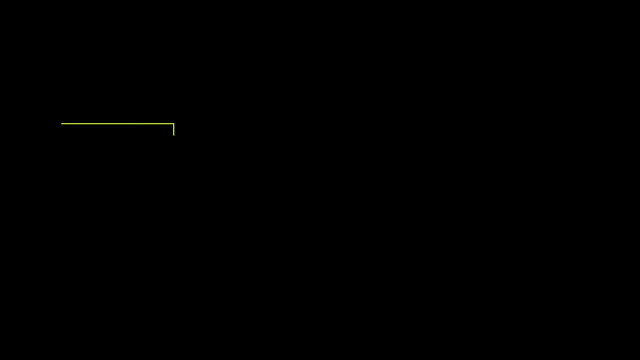 important reason to use it is that no one really knows what entropy is, so it helps in winning debates. Moral of the story: sometimes even some of the greatest engineers don't really think too hard about naming conventions, so you shouldn't either. The cool aspect of entropy is it has a 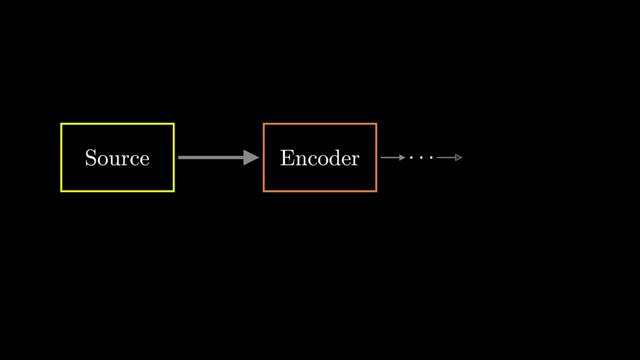 lot of implications for compression and encoding algorithms. Let's go back to the original source and receiver setup. A large focus of Shannon's work in this domain was thinking about not necessarily individual messages, as we've done so far, but more so a general set of symbols sent. 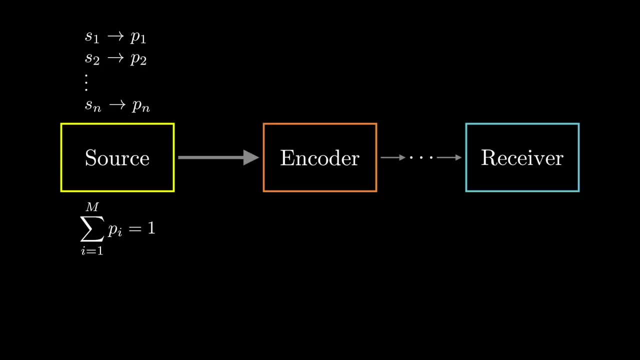 according to some distribution. One simple example is the following set of symbols where the source is equally likely to send A, B, C or D. Suppose we use the following encoding scheme: We want to have some metric to compare encoding schemes with each other and 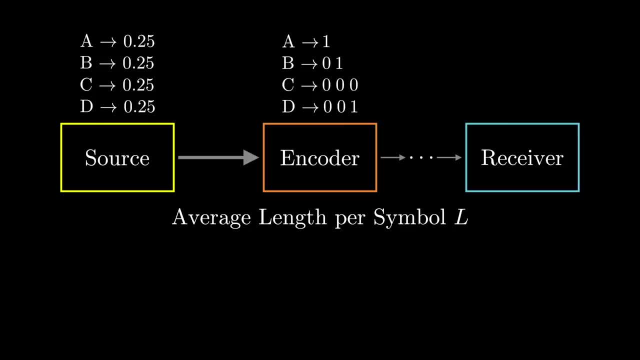 want to have some metric to compare encoding schemes with each other and want to have some. One common metric used in information theory is the average length per symbol. It's calculated by weighting the length of each symbol's encoding with the probability that the symbol is sent by the source. 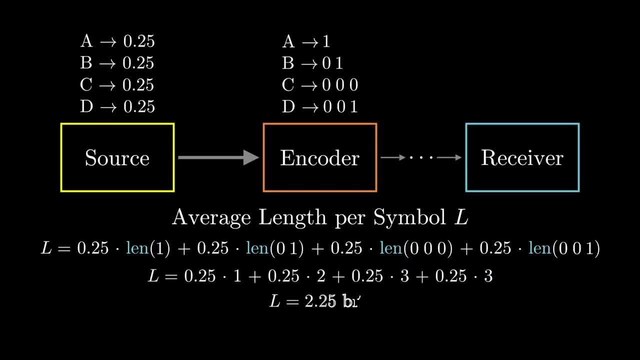 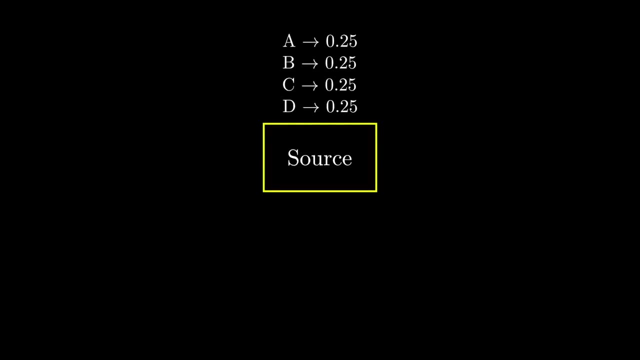 So with this particular encoding and initial distribution the average length per symbol is 2.25 bits, While with this particular distribution the average length per symbol is slightly smaller. Now here's the really interesting discovery. Let's say the source sends a message with symbols from this distribution. 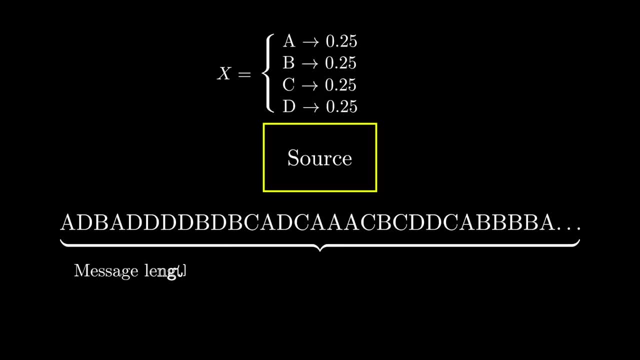 Shannon discovered that as the length of the message approaches infinity for any lossless compression method, the fundamental lower bound on the average length per symbol is the entropy of the source distribution. No matter what encoding scheme you try, you cannot reduce the average length per symbol. 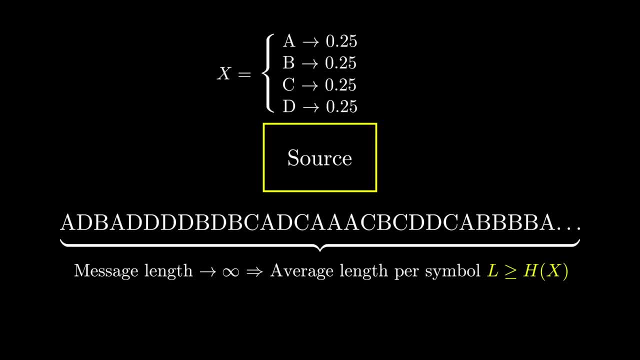 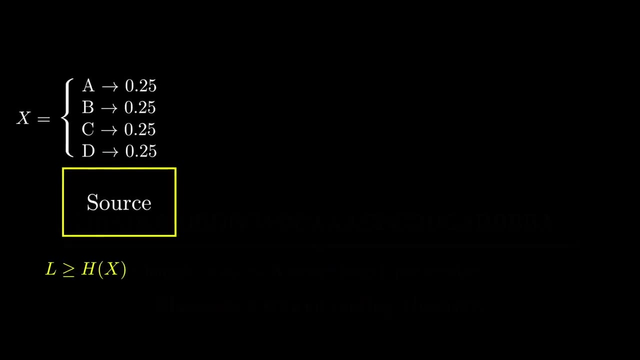 below the entropy without guaranteeing that you lost. This was a key part of Shannon's Source Coding Theorem. There is a formal proof of this theorem that relies on some more advanced concepts in information theory and I'll link it in the description. but let's get an intuitive sense for why. 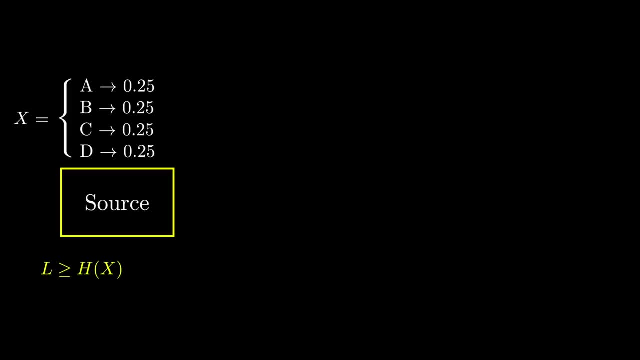 this is true. The entropy of this particular situation, when we are equally likely to send each symbol, is 2 bits. We have some theoretical understanding for entropy, but if you're like me, this number doesn't really mean anything, unless we have some notion of it. 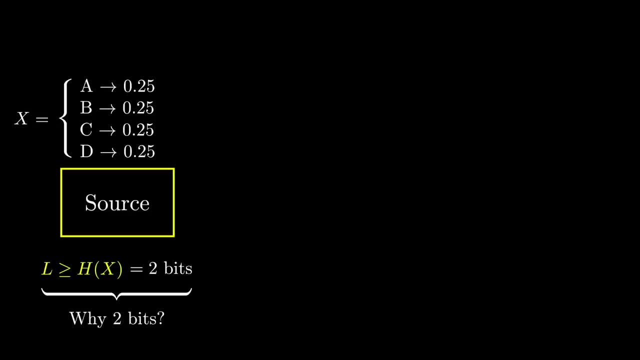 So let's get started. Let's put ourselves in the shoes of a receiver. Let's say a source sends a symbol. according to this distribution, Suppose the receiver needs to ask questions to figure out what symbol it is. What's the best set of questions to ask? 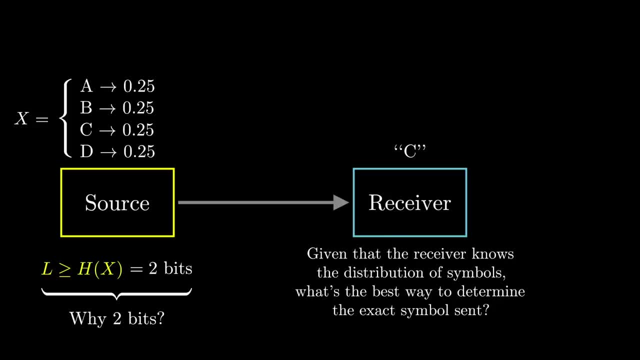 The goal here is to ask the fewest number of questions to determine the exact symbol. Here we have 4 possible symbols, all equally likely. So the first question is the lowest possible number. The second question would narrow our search to 2 symbols and then from there we can pinpoint. 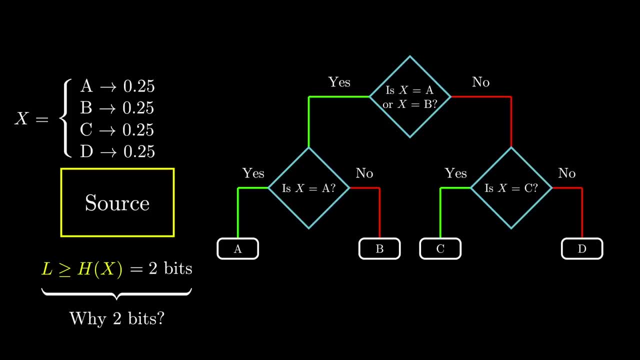 the exact symbol. Notice that the best the receiver can do is 2 questions and if we treat each yes or no response as a bit, this defines the best possible encoding scheme for a compression algorithm. The essence of Shannon's Source Coding Theorem says that you cannot do better than. 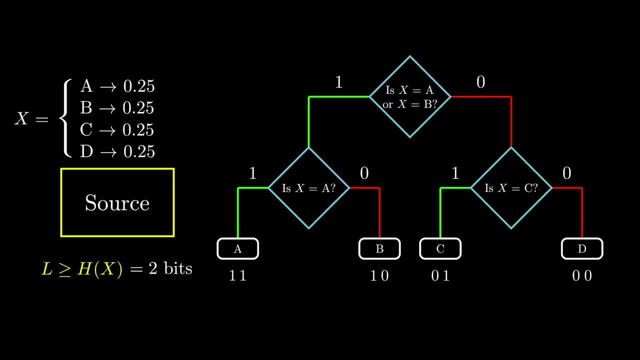 an average length of 2 bits for any encoding scheme for this particular distribution, and this diagram provides a good intuition for why that's true. When the symbols aren't equally likely, it's more interesting. We could do the same encoding scheme as before and get an average length of 2 bits once again. 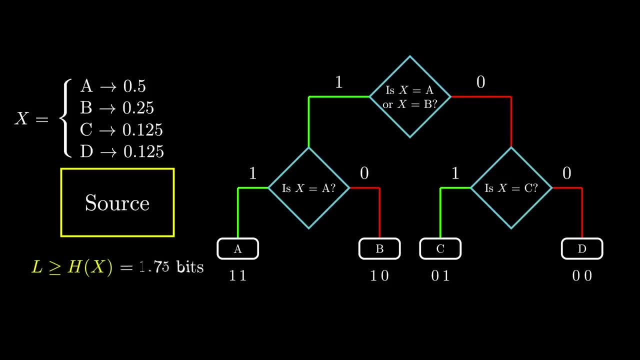 but is this really the best we can do? The entropy in this situation is 1.75 bits. Can we get closer to the lower bound? In some situations we can't, but in this case there are some inefficiencies in our current encoding. 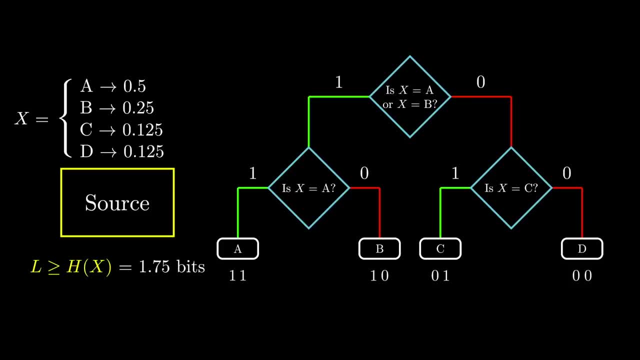 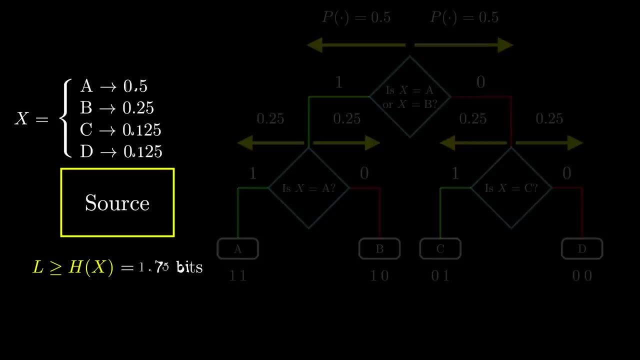 Take a second to see if you can come up with a better encoding. If you think about what we did in the situation of equally likely symbols, it all boiled down to splitting our distribution into equally likely groups. Let's see if we can try the same thing here with this distribution. 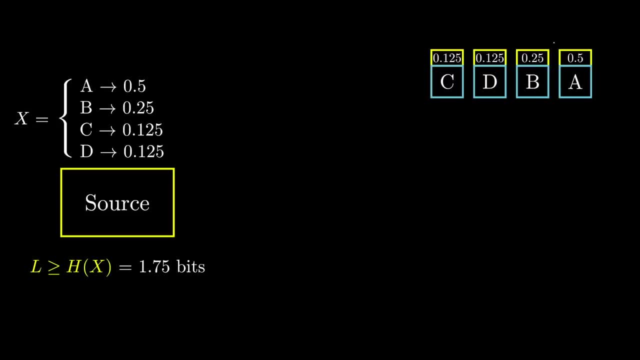 It makes sense to start off with sorting our probabilities in ascending order, where we can then find our first split On the right side. we only have one element, So we're done. The remaining work is all about splitting the left group of symbols. 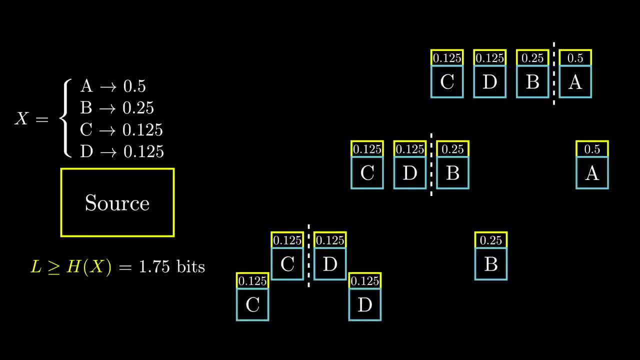 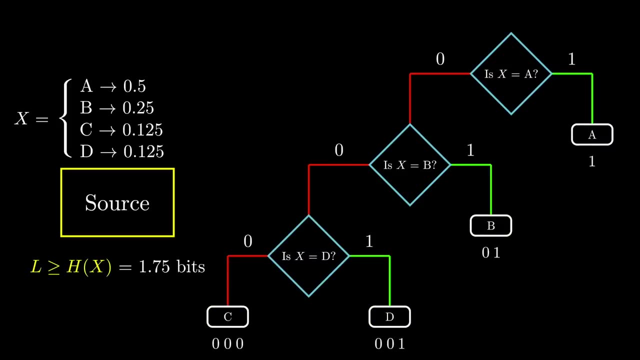 It's not too difficult to see the rest of the appropriate splits, and we continue splitting until every symbol is no longer part of a group. We can translate this easily to our earlier question diagram and from that we can get an encoding. Notice that the average length per symbol now is exactly the lower bound provided by. 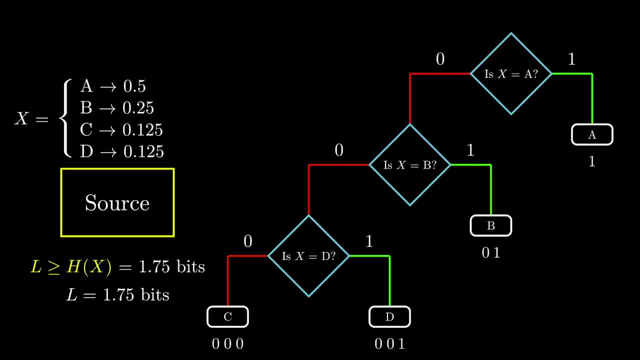 the entropy. The key idea here is that we gave more likely symbols a smaller encoding. That's a big theme in data compression. By giving more likely symbols smaller encodings, we reduce the average length per symbol and get better overall compression. One interesting coincidence here is that in our examples the entropy ended up being exactly. 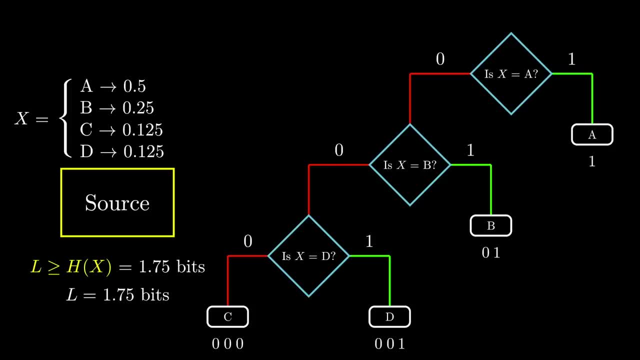 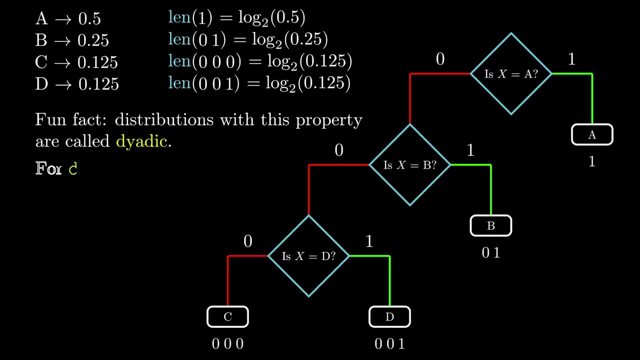 equal to the average length per symbol. The astute among you may have noticed that the distributions I picked were not exactly equal, nicely defined such that each symbol's encoding length is exactly equal to the number of bits in the self-information of that symbol. That's why, in these situations, the average length 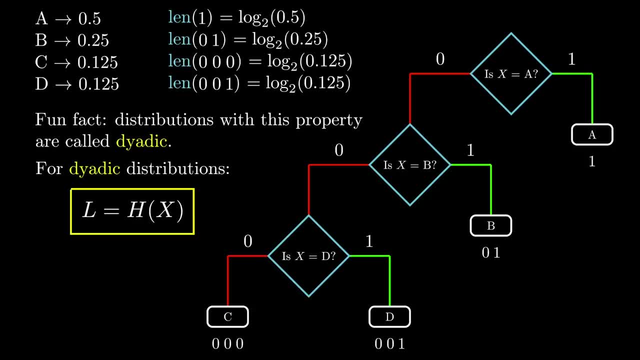 per symbol will always be exactly equal to the entropy of the distribution. So we just saw two examples of distributions where we came up with the optimal encoding, which is the goal of the original problem given to Huffman. A natural question from here is: can we extend it to any general distribution? This is exactly what both Shannon and Fano 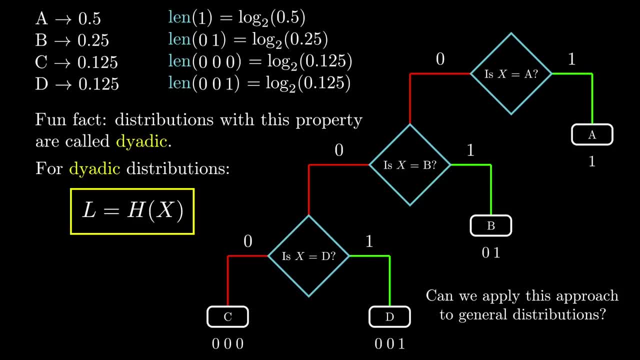 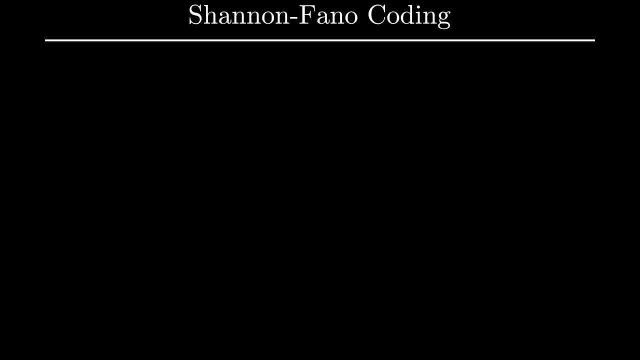 tried to do. In fact, what we did here basically inspired one of the first widely used compression algorithms proposed by Shannon and Fano, which they aptly named Shannon-Fano coding. When you invent fields like information theory, you can basically name everything after yourself. 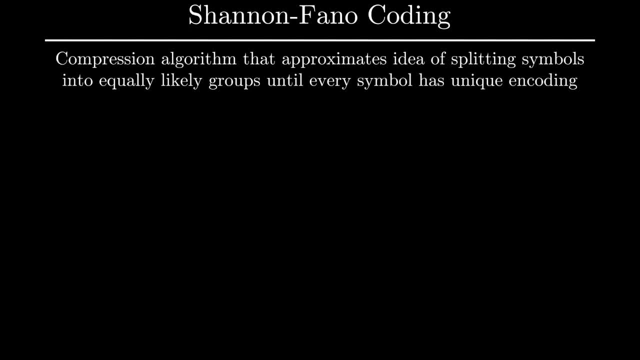 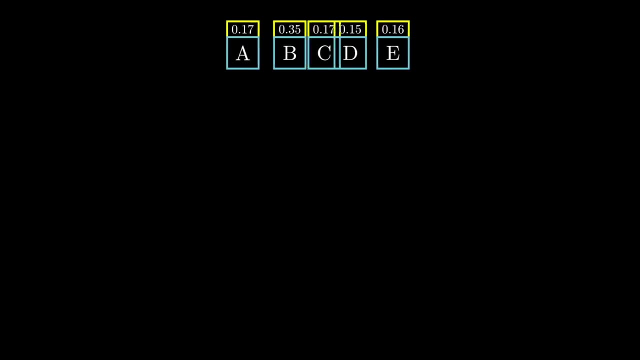 Shannon-Fano coding attempts to approximate the idea of splitting our symbols into equally likely groups, and by doing so we can get the same result. I find it easiest to understand with an example. Given these probabilities, the first step in Shannon-Fano encoding is to sort the probabilities in increasing order. 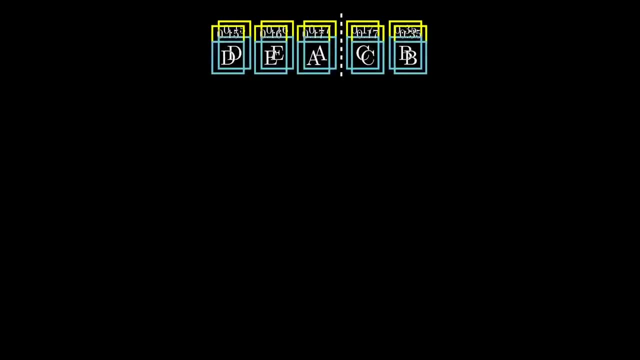 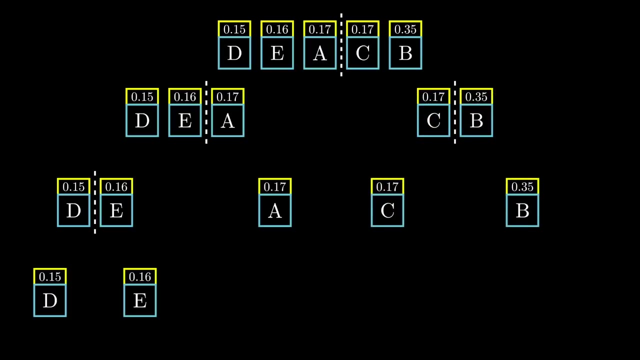 We find the best split of probabilities between the two groups, such that the sum of each individual group is as close to each other as possible. It then repeats the same process recursively on each group until every group has one. The encoding is simple: once we have the splits, Every time we go to the left group. 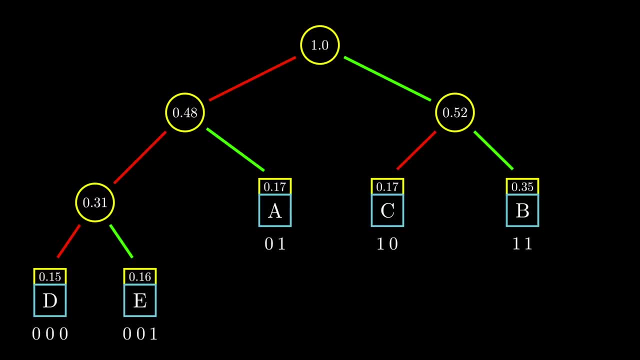 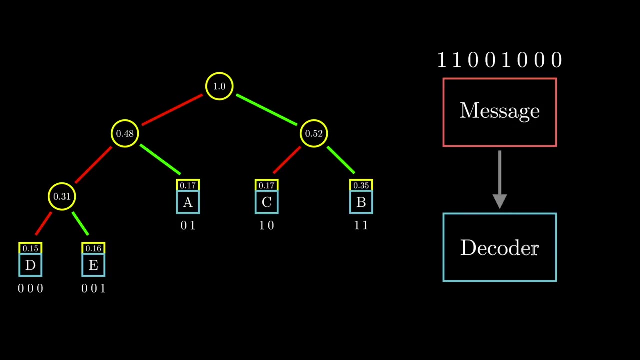 we add a zero and every time we go to the right we end up with the one. One nice aspect of this algorithm is by using trees. every code has a unique path in the tree, so when we put this together in an encoding for a message, there is no ambiguity for a decoder. 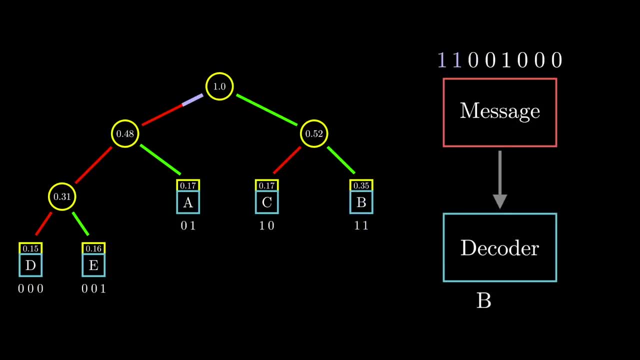 Decoding boils down to just traversing down the tree until we find a symbol, going left if we encounter a zero and going right if we encounter a one. The types of codes that Shannon-Fano encoding produce are often called prefix-free codes. 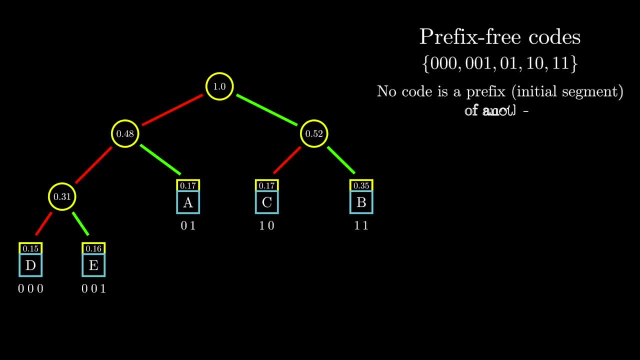 since no code is a prefix of another code, They can always be represented by a full binary tree, such as this one, where every node has either zero or two children. This is a key property we'll come back to, so keep it in mind. 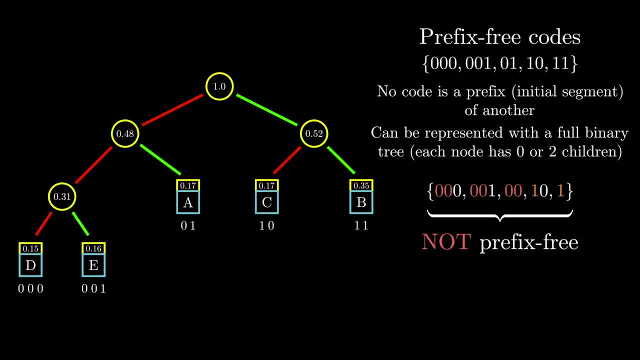 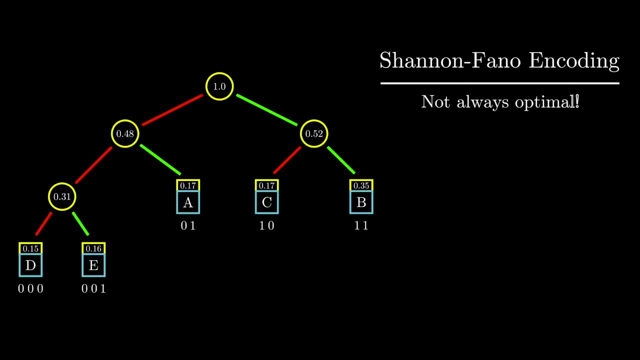 For a couple years, Shannon-Fano coding was the best scheme people had to perform lossless compression and it produced optimal codes for a variety of distributions. However, Shannon-Fano coding does not always produce an optimal encoding, meaning there sometimes exists another encoding scheme with better average length per symbol. 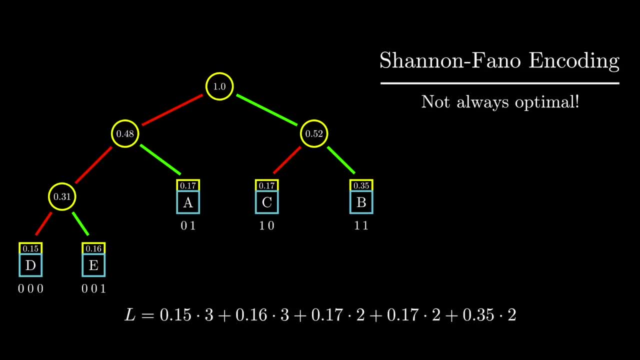 For example, on this particular distribution, Shannon-Fano coding produces an average length per symbol of 2.31 bits, But the scheme that Huffman came up with, which is always optimal, provides the following encoding, which just barely beats Shannon-Fano encoding: 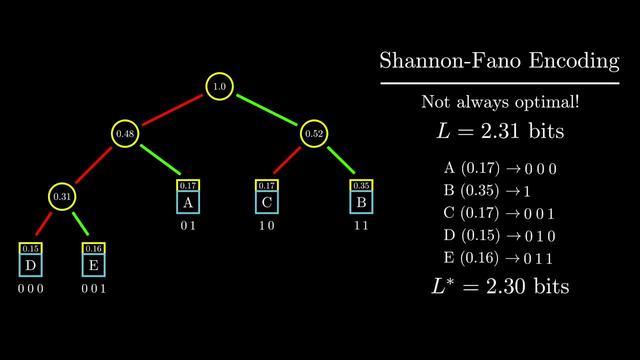 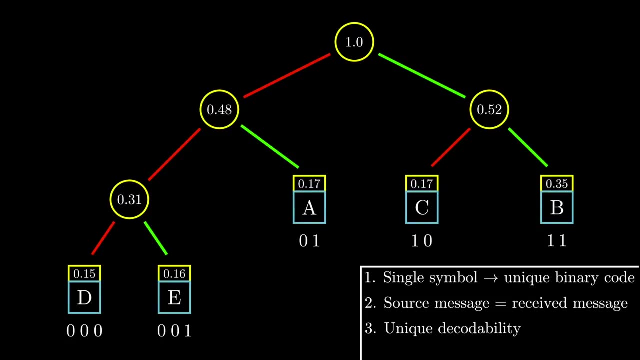 The question now is how in the world did Huffman find a better algorithm that both Shannon and Fano missed? Let's take a step back and revisit the requirements of our original problem. We had three central requirements and we see that Shannon-Fano coding does satisfy. 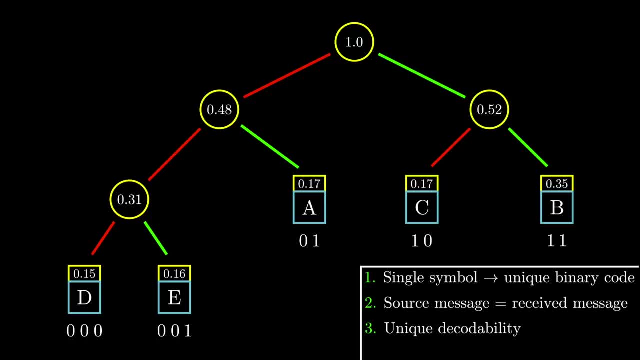 these requirements by its use of prefix-free codes and full binary trees, and Shannon-Fano coding does satisfy these requirements by its use of prefix-free codes and full binary trees. Now the additional constraint we want when dealing with optimal compression is: we want our encoding to have the minimum possible average length per symbol. 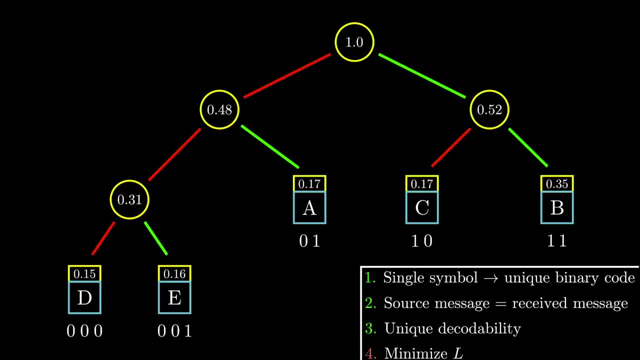 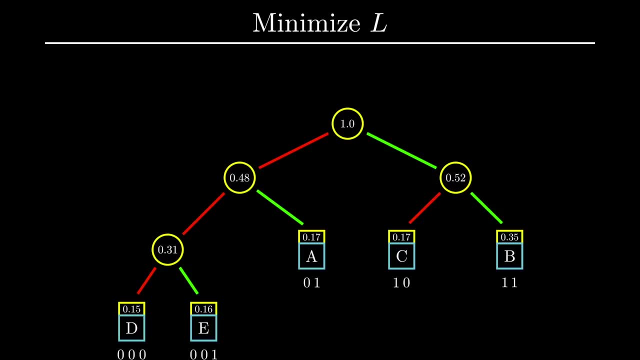 We just saw an example of how Shannon-Fano fails here, so let's dive deeper into this requirement and see how we can come up with something better. Since Shannon-Fano encoding solved a lot of our requirements, let's use the framework it provides to figure out how we can improve upon the average. length per symbol. Since Shannon-Fano encoding solved a lot of our requirements, let's use the framework it provides to figure out how we can improve upon the average length per symbol. Since Shannon-Fano encoding solved a lot of our requirements, let's use the framework it provides to figure out how we can improve upon the average length per symbol. 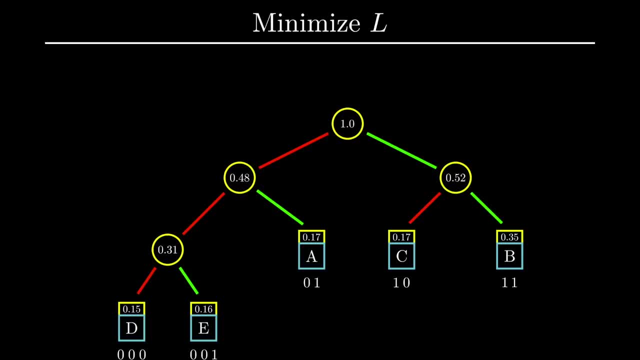 When using full binary trees to represent prefix-free codes. one nice way to calculate the average length per symbol is by using the depth of the tree, since the depth of the tree corresponds exactly to the encoding length. What does this formulation immediately imply? One immediate fact that comes from this formulation is: it must be true. 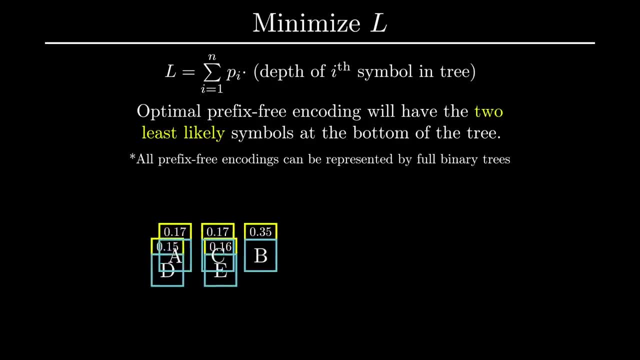 that the optimal full binary tree representation must have the two least likely symbols at the bottom of the tree. In other words, it can never be the case that there exists some other symbol in the optimal tree that has longer encoding length than the two least likely symbols. 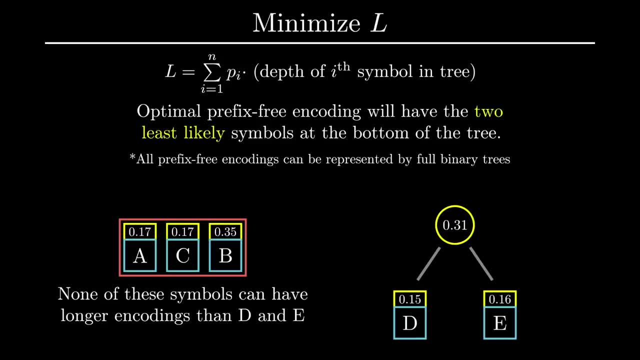 This makes sense intuitively, since we want less likely symbols to generally have longer encodings, But this is powerful. What this implies in general is that, given any set of symbols we can take, the two least likely symbols create an internal node. that's the sum of their probabilities. 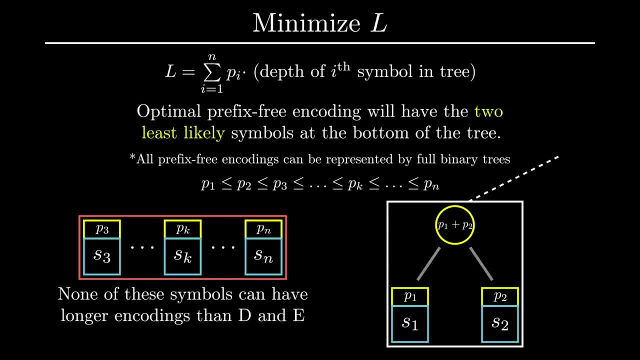 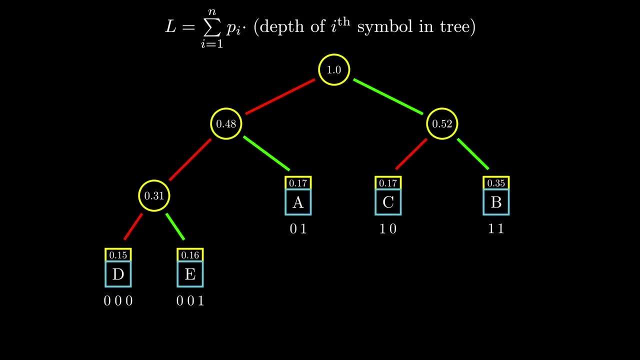 and this subtree is guaranteed to be part of the optimal tree. Now the question is: how do we construct the rest of the optimal tree? This is where something pretty clever and by no means obvious comes into play: This formulation of the average length per symbol using the depth of the bottom node. 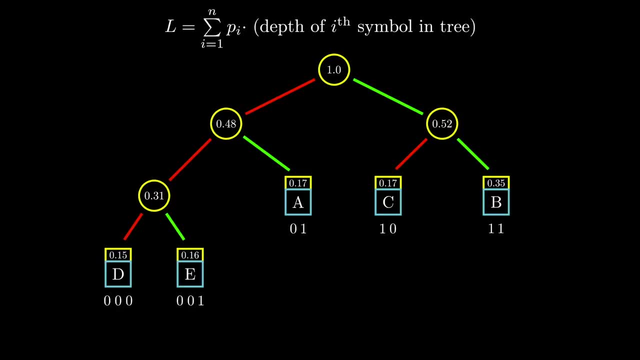 in the tree is useful and fairly clear, but there's actually one more method that works. One nice aspect of how these trees are built is: the average length per symbol is the sum of the probabilities of each node in the tree except the root. Why is this true? Let's compare this with our earlier calculation. 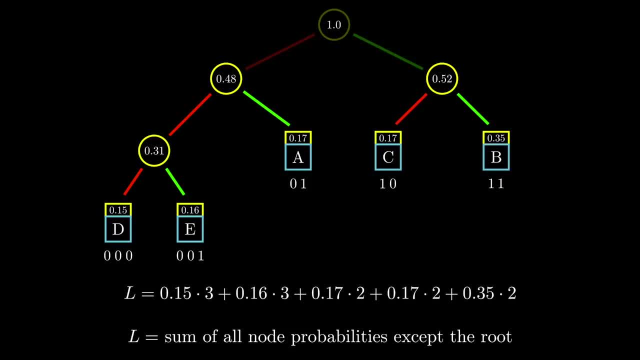 The best way to see why this is true is by expanding the internal nodes as the sum of the individual probabilities they represent. Notice that when we sum over all the internal nodes, each symbol probability gets included exactly the same number of times as the sum of all the internal nodes. 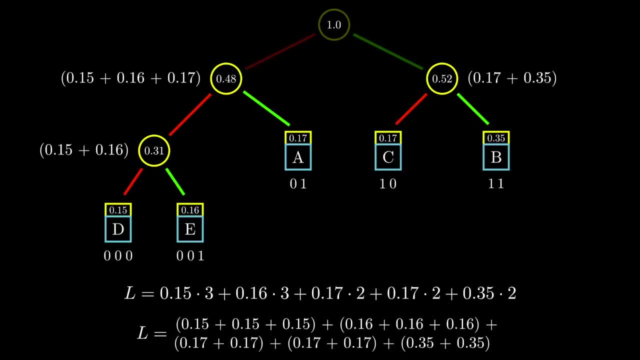 The tree has its depth in the tree, so the two formulations will always be equal. There are formal proofs of this fact that aren't too difficult to construct based on this idea, but this is a nice way to get the intuition for why it's true. 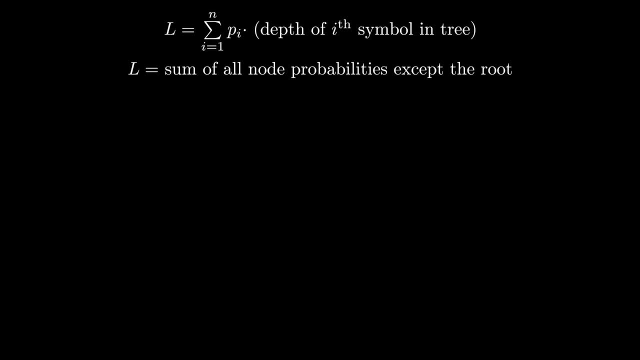 Alright, so how does this formulation help us? Let's try to be as general as possible In both of our formulations. notice that the average length per symbol is entirely a function of the probabilities, since the probabilities of symbols determine the optimal encoding. 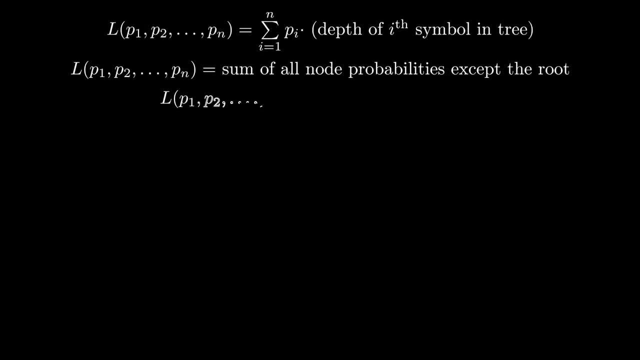 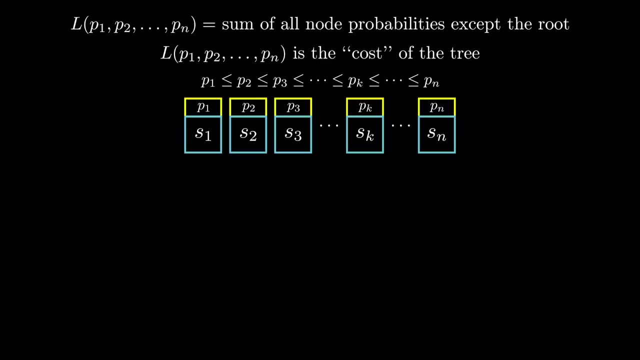 and, as a result, the optimal tree. Our goal is to minimize this function for a general set of symbols with a defined probability distribution. I'll refer to this function as the cost of our tree. We know from earlier that our optimal tree will for sure have the two symbols with the 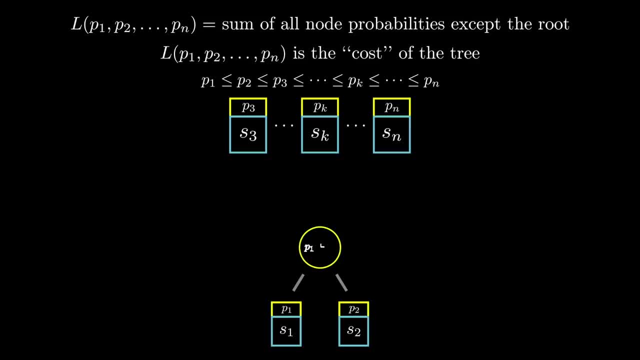 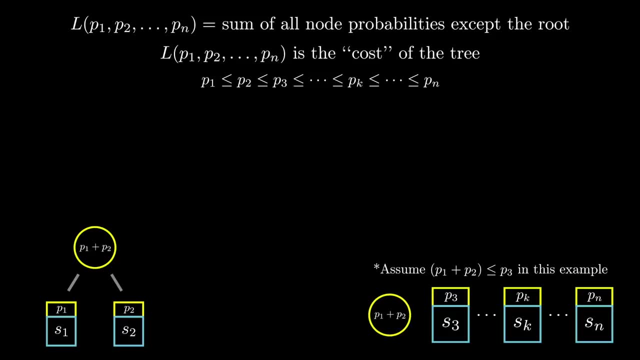 smallest probabilities at the bottom of the tree, which ends up creating a new node. Let's add the new node to our set of nodes that we need to process. Now here's the cool part: Using our new formulation, where we take the cost of our tree as the sum of all nodes in the tree except. 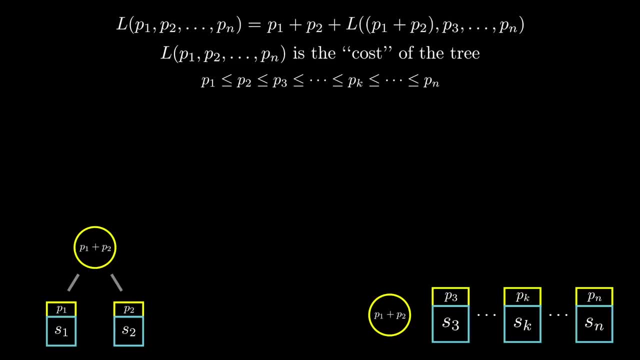 for the root. the cost can be reformulated as the sum of the two smallest probabilities and the cost of the optimal tree containing this new internal node as a leaf and all other symbols with their respective probabilities. In a sense, you can think of this as a way of 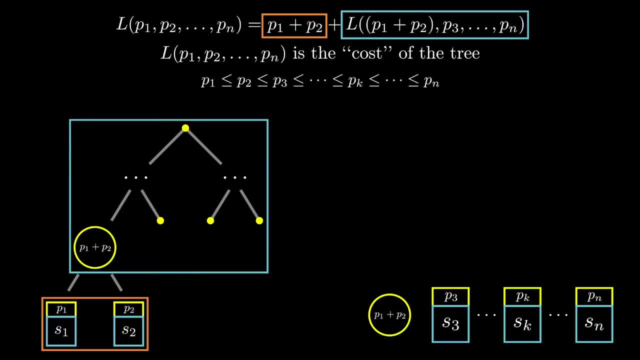 separating these two bottom nodes from the rest of the tree For an optimal encoding. the rest of the tree is the optimal tree for a given set of n-1 nodes with this probability distribution, And the beautiful thing here is that this problem is really just a smaller version. 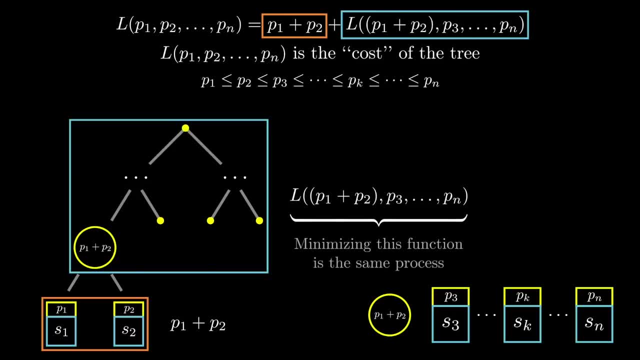 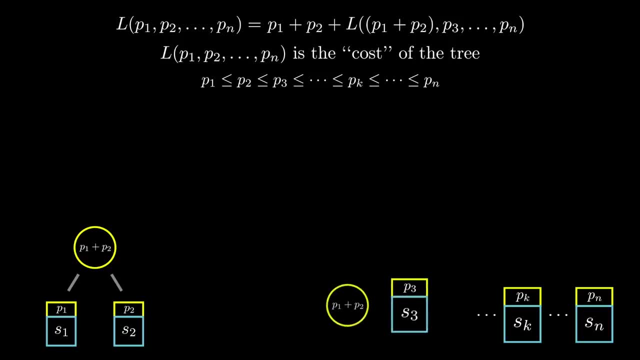 of our original problem. The way we minimize this particular cost function is the exact same process. We can take the smallest two probabilities from this set and make a new internal node from those two probabilities and continue building the tree in this fashion. This is the essence of the Huffman encoding algorithm. Let's put this all together and show. 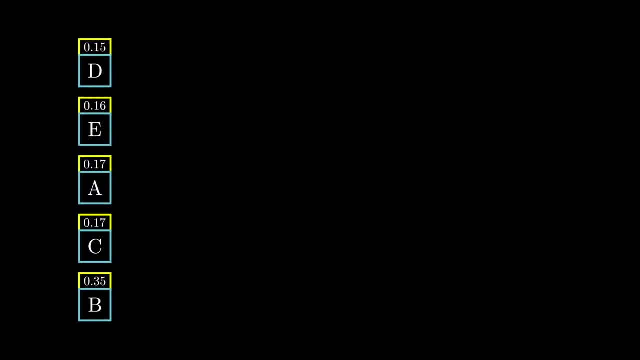 how this works. on the example we've been looking at thus far, We start off with the two lowest probability symbols, making a new internal node with the sum of these two probabilities. Now the key finding is we have to repeat the same idea, but now on a set of three symbols and this new 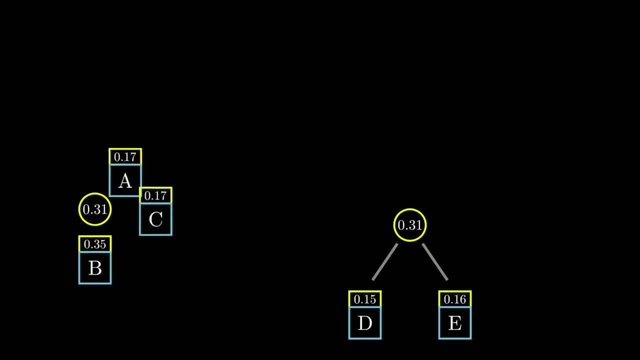 node with probability 0.3.. We once again pick the two lowest probability elements and make a new internal node, as we did before. The key idea here is that these two internal nodes are guaranteed to be part of the optimal tree. Now we have two internal nodes left, along with one symbol: The elements. 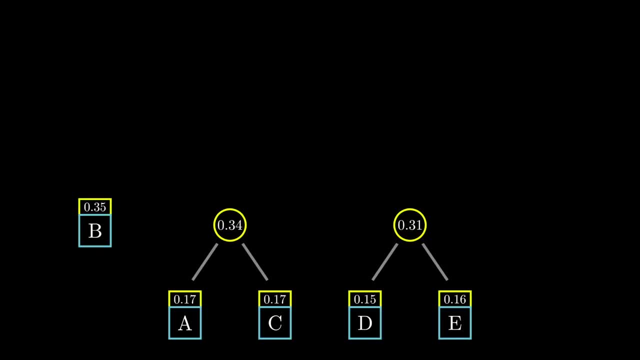 with two lowest probabilities are the internal nodes. so we make a new node with the sum of these two internal nodes. We now have two remaining elements, one a node and another a symbol. This means we can take them and create the root of our tree. 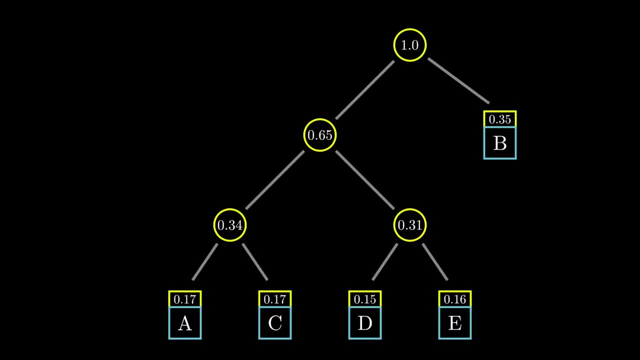 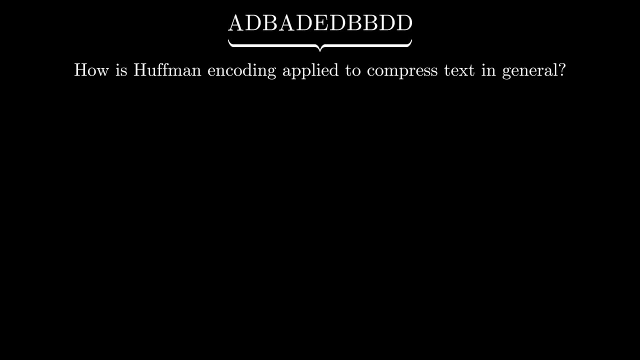 and that right there is the Huffman tree with the guaranteed optimal encoding for this distribution. One question I'm sure has been on your mind is how this applies to real-world compression of text. So far we've been looking at this algorithm from a fairly theoretical perspective, but in practice, 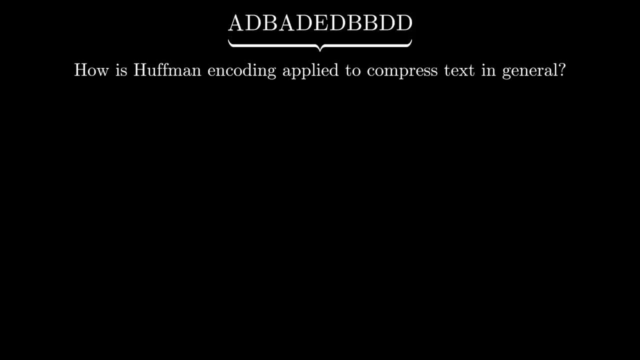 we'll just get some text with no associated probability distribution, But fortunately we can still use Huffman. Instead of thinking of symbols with associated probabilities, we will use the frequencies of characters to determine the encoding, with higher frequency characters generally having the fewest bits in their encoding. Once you have the counts of each. 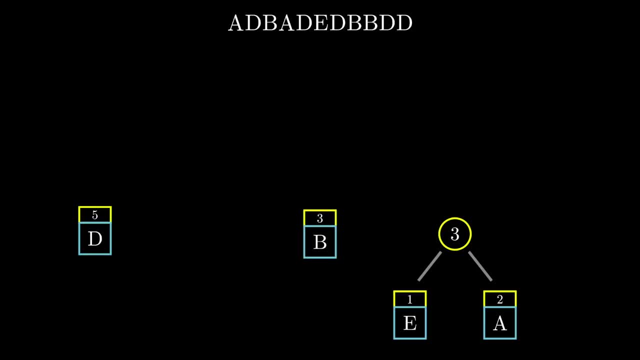 character in a text file. Huffman encoding is the exact same process as before. The two lowest frequency characters are continuously used to make new nodes until we have the entire Huffman tree. Let's talk about the implementation of Huffman encoding, The specific part of the implementation. 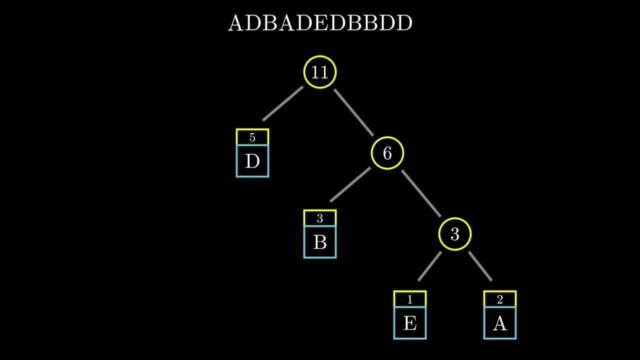 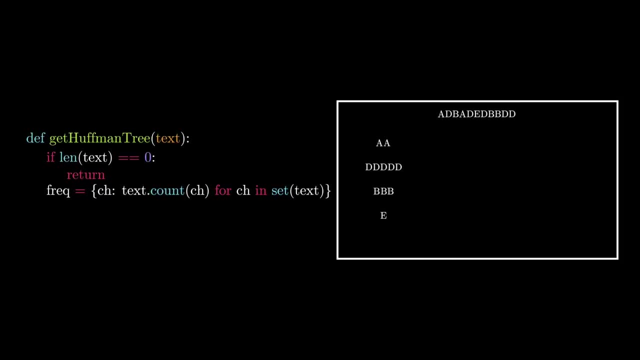 we will discuss is how we build the Huffman encoding tree. Given some text, the first set of information we need is the frequencies of each character in the text. Then, for our tree, we want to define a node class that stores each character with the relevant 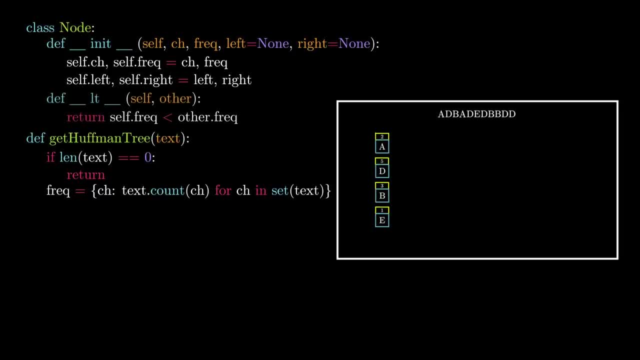 frequency. We also want to implement a way to compare nodes, since that's one of the core parts of optimal encoding. The key implementation detail here is that one of the simplest ways to implement Huffman encoding is by using a priority queue. A priority queue is a handy 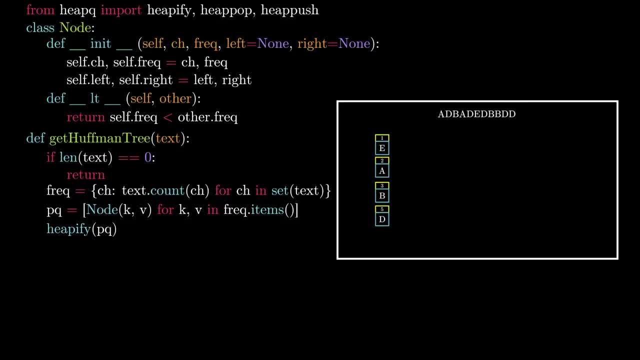 data structure that efficiently keeps track of the minimum element in a collection of elements. Using a priority queue makes it easy to continuously remove the two smallest elements, form a new node from these elements and then insert the new node into the queue CONCLUSION. At the end, the node will be less than 1.5mm high from the previous row. 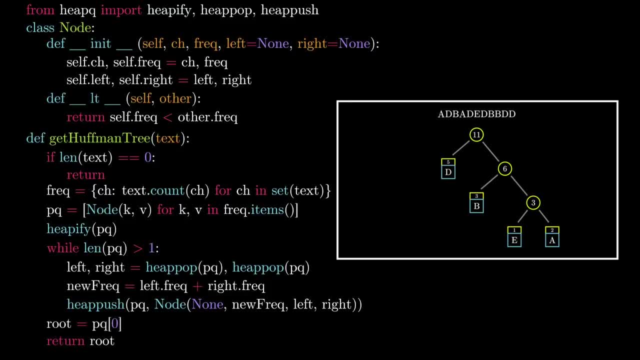 and the data structure will be less than 50mm higher from the previous row, So we want to create a space that contains all of the P eq of the vector that we wanted to throw. This is designed for encoding To use this style, And the last element in the queue ends up being the root of the Huffman encoding tree. 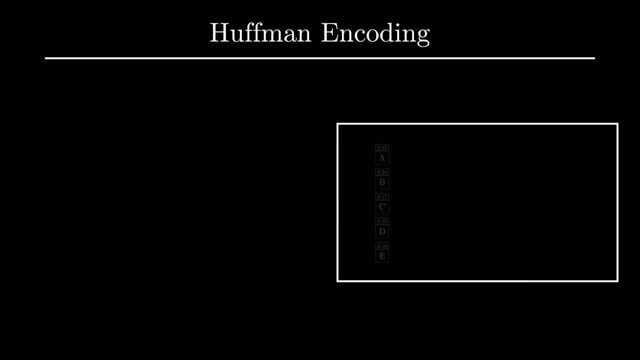 So there you have it, that's Huffman encoding. Not only is it the optimal encoding algorithm under the given constraints, it's surprisingly simple and elegant, So much so that, in retrospect, looking at the Huffman encoding algorithm, it's easy to think: hey, that's kind of obvious, right. 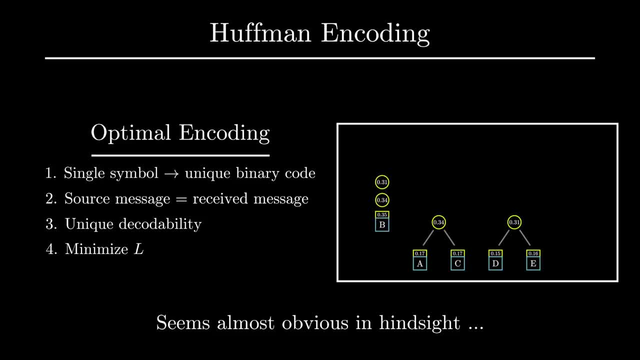 Of course, we should take the least likely symbols and give them the smallest encoding and then build the tree up from there, and I think, to an extent, when you first encounter this algorithm, that's a common thought process. But remember, some of the world's best minds in information theory were stumped over this. 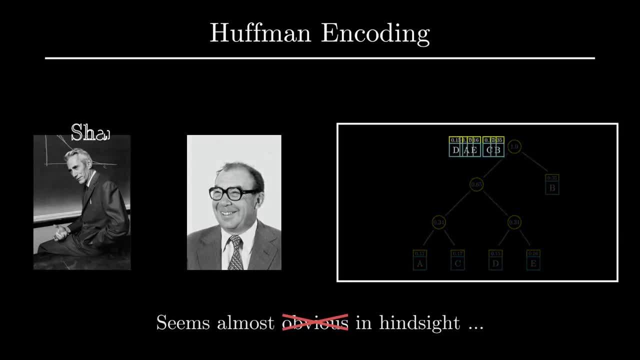 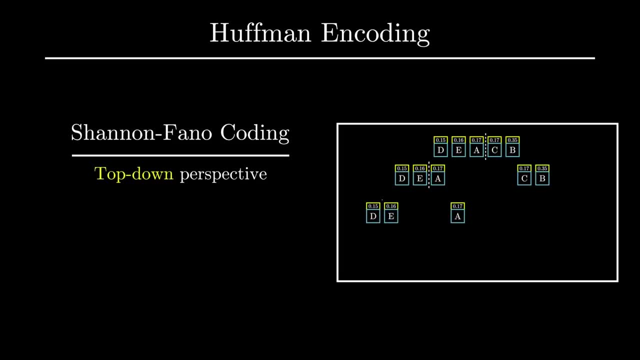 very problem. The predominant compression method before Huffman encoding was Shannon-Fano coding, which looked at this problem from a top-down perspective when we tried to optimally split symbols into groups, And a lot of times this works quite well and produces the optimal encoding. 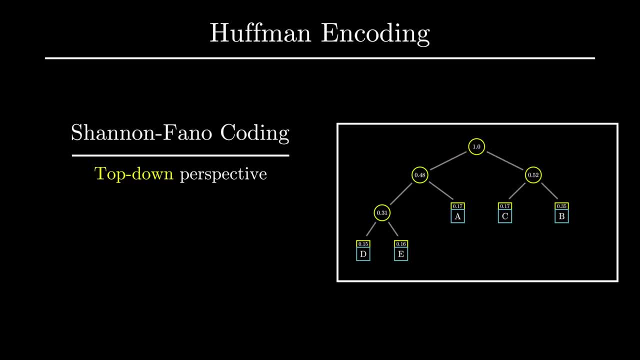 But to guarantee optimality. the cool shift in perspective that Huffman came up with was to look at building the tree from the bottom up. The smallest shift in perspective can sometimes make all the difference. I'll freely admit that the way we covered Huffman codes in this video is definitely 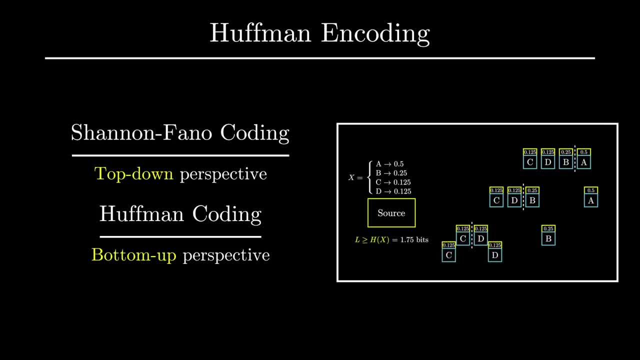 not standard. In fact, when I first learned Huffman codes, it was within the context of an algorithms class that mentioned it as an example of a greedy algorithm. It wasn't until I saw it in an information theory context that I gained a true appreciation for it. 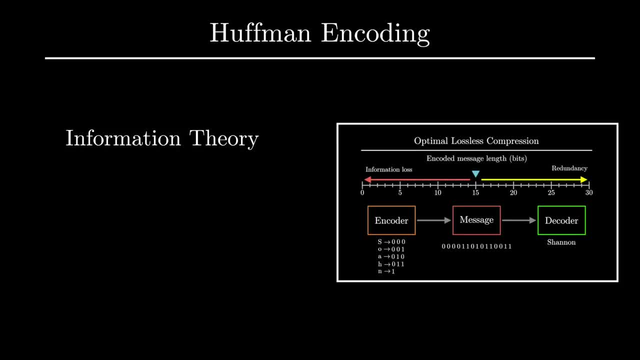 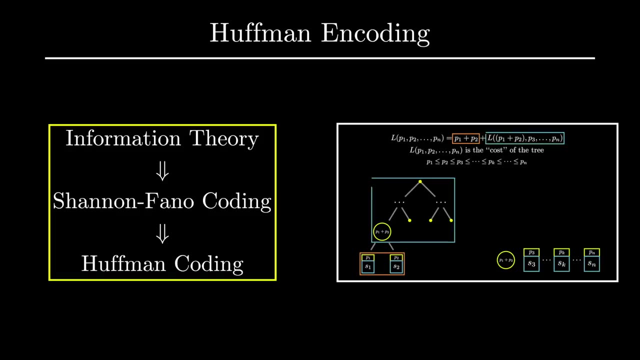 If we look back on the story here, it all started with the fundamentals of information theory, which directly motivated Shannon-Fano coding Huffman then provided the key improvement that guaranteed optimality. Seeing how this all comes together is just immensely satisfying to me.